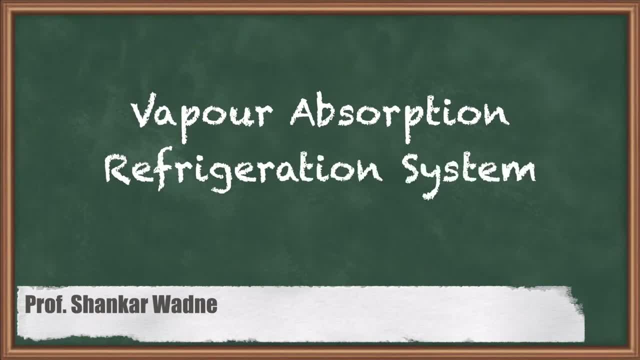 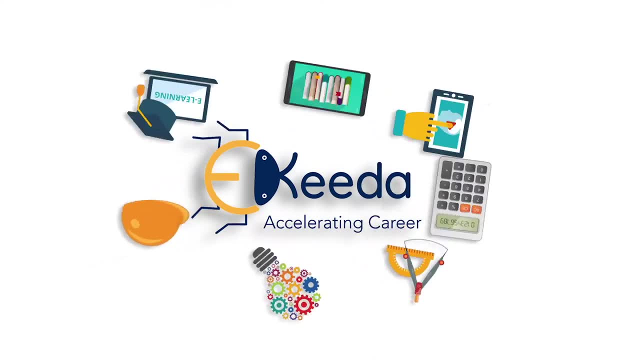 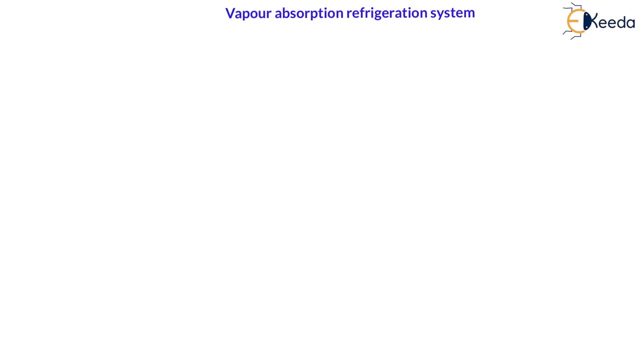 Hello, my dear students, in this lecture we are going to see one of the topic of refrigeration, that is, vapor absorption refrigeration system. Now, this vapor absorption refrigeration system is also represented as VARAS. that is, vapor absorption refrigeration system. Now, my dear students, in previous lectures we have seen 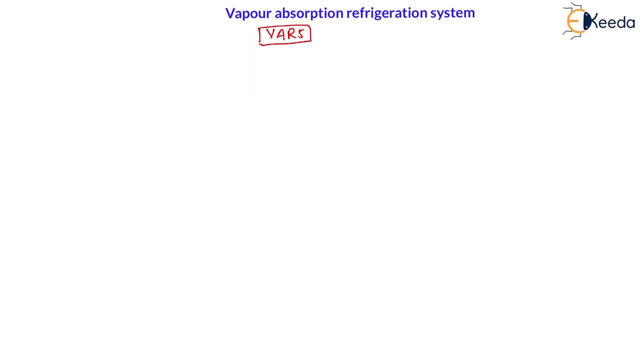 vapor compression refrigeration system, which is also called VCR, vapor compression refrigeration system. Now, my dear students, in case of vapor compression refrigeration system, we have used compressor for compressing the vapor, But here, in case of vapor absorption refrigeration, 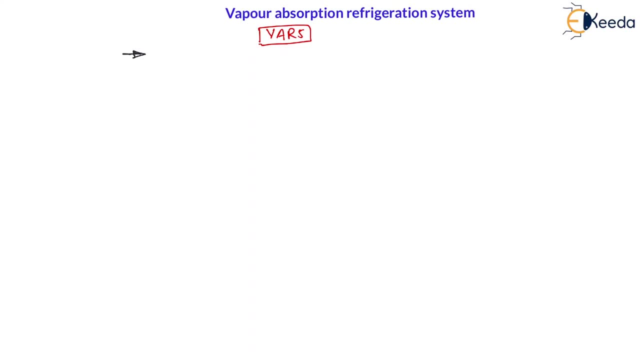 system, vapor is absorbed, Means. here there is no need of compressor. Here no need of compressor, No need of compressor As vapor is absorbed, As in this case, vapor is absorbed, Vapor is absorbed. This is the very first point regarding vapor compression refrigeration system: vapor absorption refrigeration. 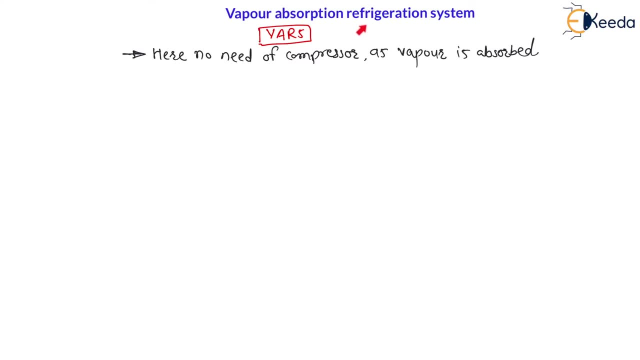 system. Now, in case of vapor compression refrigeration system, compressor was used. And, my dear students, compressor works on the electricity And compressor consumes lot of electricity. And here, in case of vapor absorption refrigeration system, this compressor is not used because 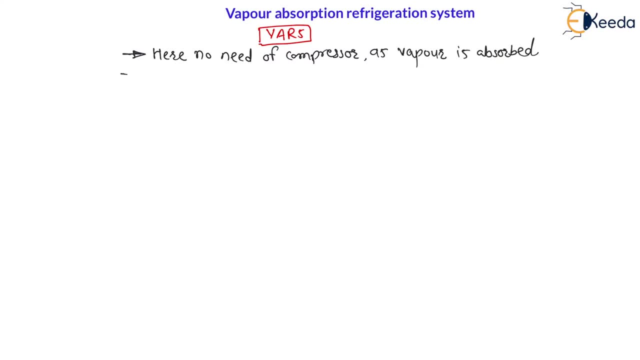 here we are absorbing the vapor. So, my dear students, the second point regarding vapor absorption refrigeration system is this system- This system means vapor absorption refrigeration system- is used. VARAS is used where the cost of electricity, cost of electricity, comes in the form of VARAS. VARAS is used where the cost of electricity is high. Now, my dear 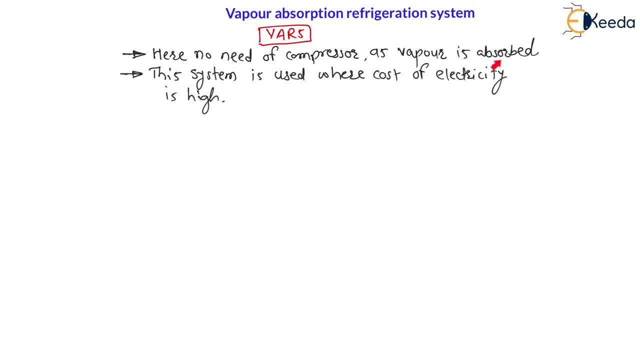 students, as we are replacing this compressor with absorption device. therefore, here the electricity consumption will be less. in case of vapor absorption, refrigeration system And hence, as electricity consumption is less so when your cost of electricity is high, this system is beneficial Because this will reduce the electricity cost Right And my 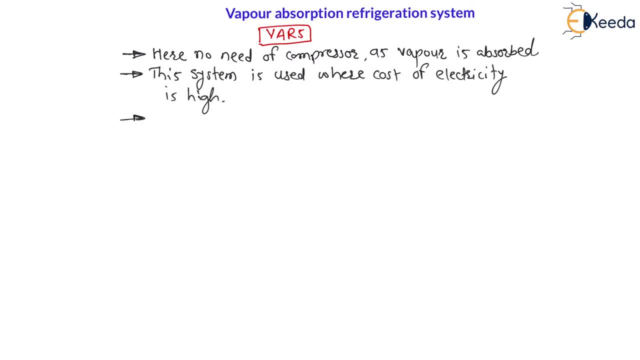 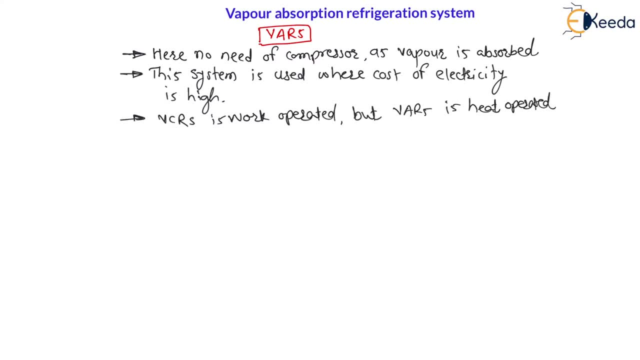 heat operated. Right Means in case of vapor compression refrigeration system, we need a work of compressor and which is useful to calculate the COP of cycle. But in case of vapor absorption refrigeration system, it is a heat operated. There is no work Right. 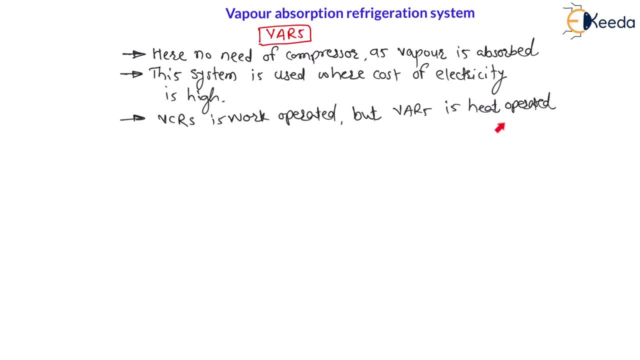 Means. the COP is obtained with the help of heats only, That is, heat of evaporator and heat of generator. that we will see later, Right Now here. the next point regarding vapor absorption refrigeration system is that this system is used where lot of heat waste. 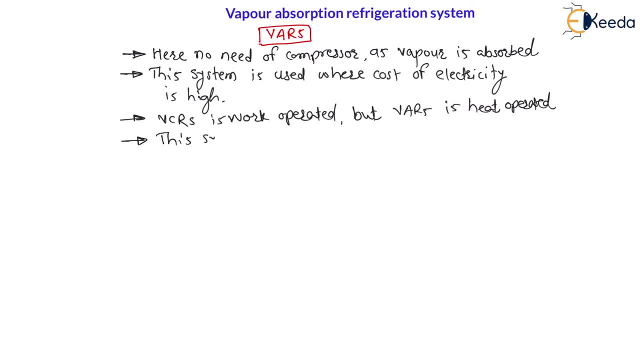 is available Right This system. we can see that this system is used where lot of heat waste. This system means vapor absorption refrigeration system- is used. is used where where lot of waste heat. Lot of waste heat is available. Is available Right As it is. 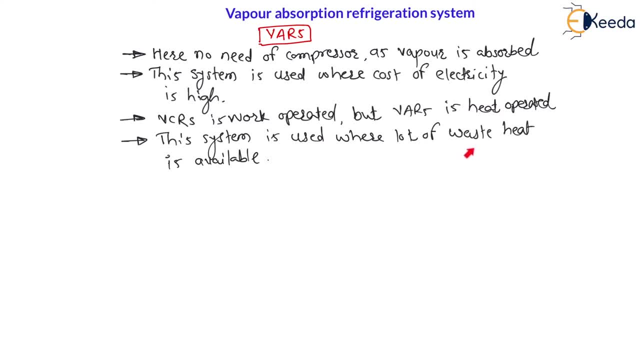 heat operated system. therefore, whenever lot of waste heat available, we can go for vapor absorption refrigeration system, For example. if you think think solar refrigerators are, For example, all solar refrigerators work on the principle of vapor absorption refrigeration system. 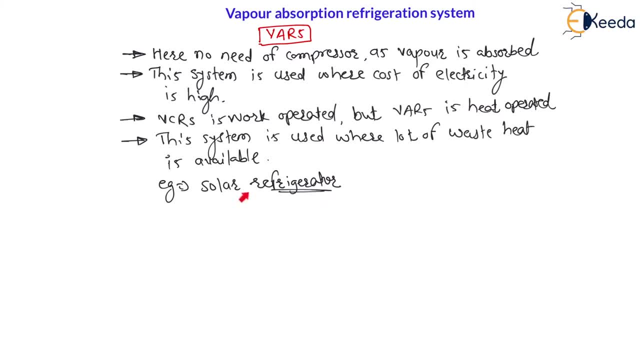 Now, my dear students, in case of solar refrigerators, they are operating on the solar energy, and sun energy is available in bulk Means. lot of solar energy is going wasted. Therefore, this solar energy is used for the refrigeration Means. solar energy is nothing but solar heat. 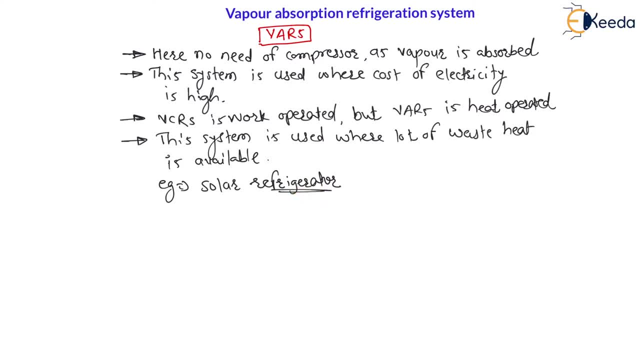 Therefore, this solar refrigerators functions on the principle of vapor absorption refrigeration system. Now, here, as in vapor absorption refrigeration system, the compressor is not used. So, my dear students, in case of VCR vapor compression refrigeration system, we are using compressor. 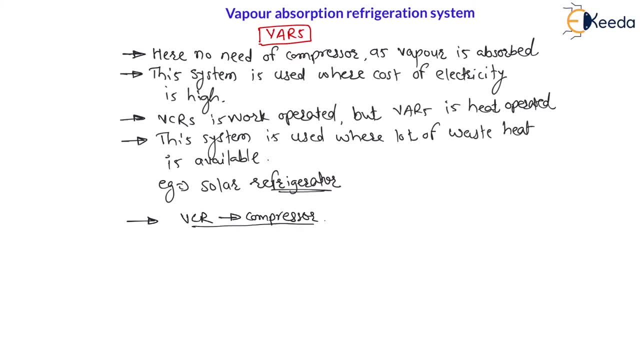 Now this compressor in case of VCR is replaced. This compressor, in case of VCR is replaced. In case of vapor absorption refrigeration system. this compressor is replaced with three devices. That is very. first device is absorber, second device is pump and third device is generator. 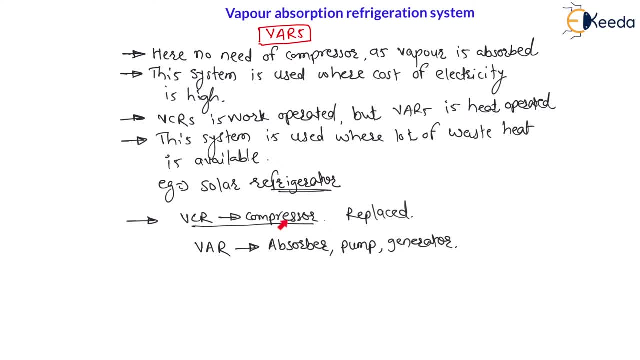 Third device is generator. Means, my dear students, the compressor of VCR system is replaced by absorber, pump and generator in case of vapor absorption refrigeration system. Right Now, already in previous lectures we have seen vapor compression refrigeration system- 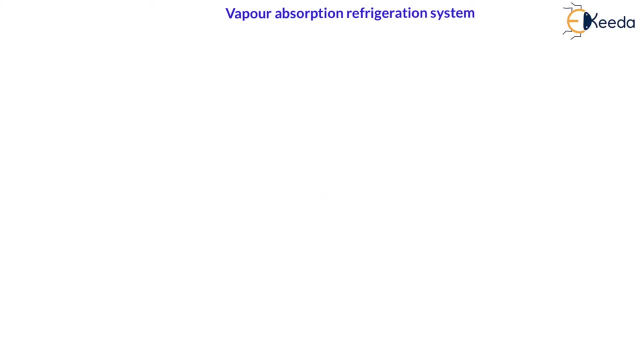 Here quickly I will draw the block diagram of vapor compression refrigeration system. And in case of vapor compression refrigeration system, the compressor we will replace with absorber, pump and generator So that we will get vapor absorption refrigeration system. 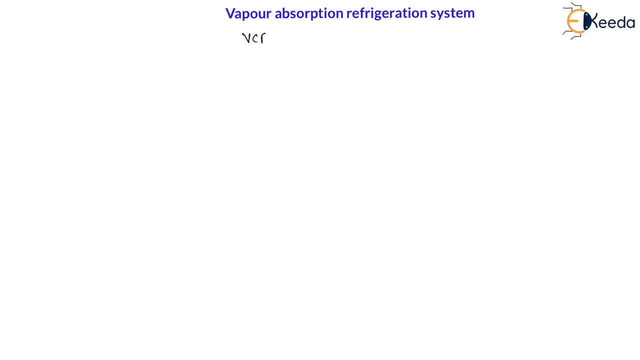 So, my dear students, in case of VCR cycle vapor compression refrigeration system, we have seen that there is an evaporator, There is a evaporator, There is a evaporator, There is a evaporator, And this evaporator is nothing but constant pressure heat absorption. 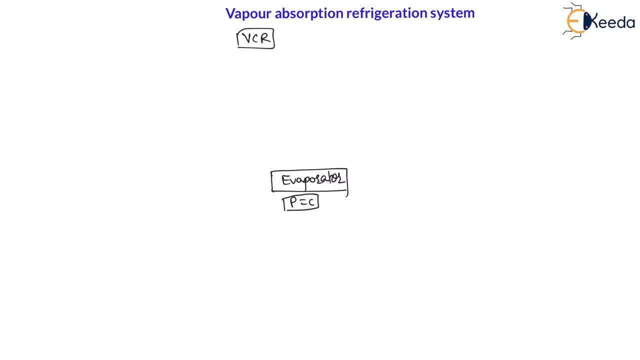 Right, It is constant pressure. Heat is absorbed Means in this evaporator. only net refrigerating effect is obtained Right After evaporator the condition was 1. And here we have given this condition to the compressor, So we have used compressor. 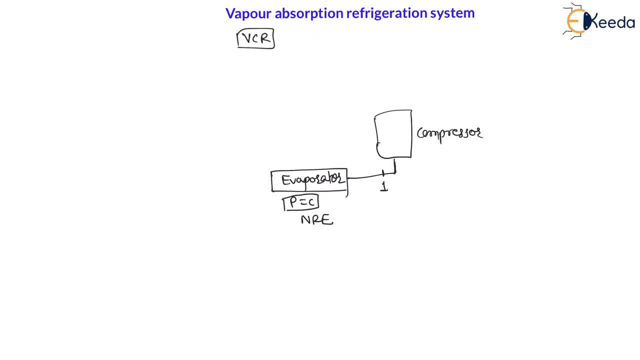 Now there will be a compressor, Right Compressor, And in this compressor the exhaust of evaporator is compressed reversibly, adiabatically, right from 1 to 2.. Right, Therefore, in compressor it is the compression is reversible, adiabatic, and compressor is electricity consuming device. right. 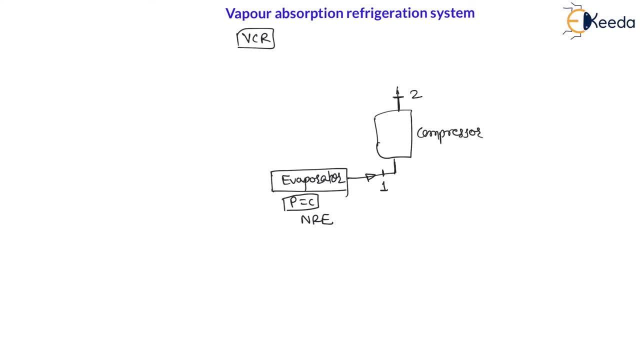 Now the exit of compressor is given to the condenser. Now the exit of compressor is given to the condenser. And again, this condenser is constant pressure heat rejection process. In condenser, at constant pressure, heat is rejected to the surrounding. 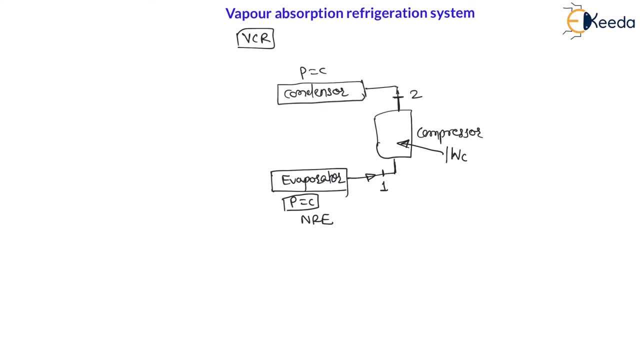 And my dear students. this compressor will consume work of compressor, That is, electricity Right And COP of the cycle. the COP of VCR cycle was net refrigerating effect divided by work of compressor. That already we have seen Because it is a work operated device. 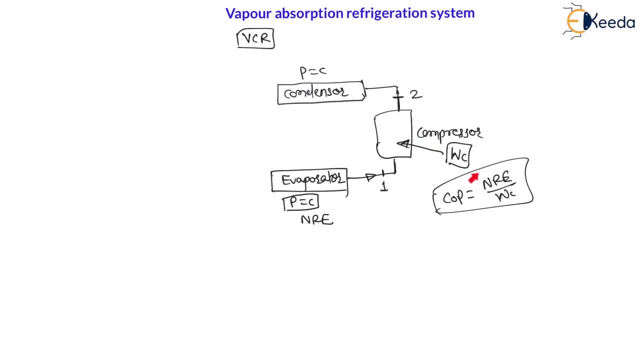 Here VCR cycle is work operated device, Because here input given is work Right. Work of compressor is the input given. Now, after compression, there is a condenser, where in condenser, at constant pressure, heat is rejected to the surrounding. 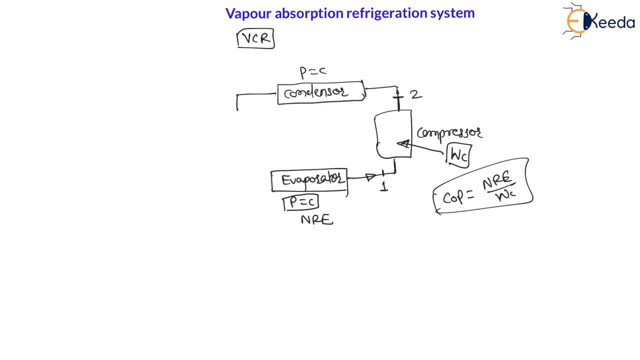 Now, after condenser, there was a throttle valve. Here there was a throttle valve, throttling device Right. Therefore, 2 to 3, there is a condenser and 3 to 4, there is a throttling. 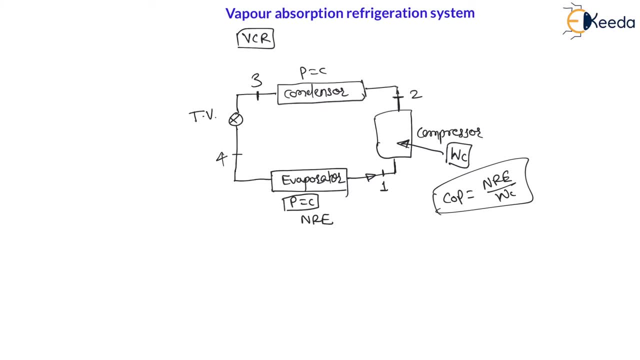 And my dear students. 4 to 1,. again there is a evaporator. These are the 4 devices in case of vapor compression refrigeration system, That is, evaporator in evaporator, we will get net refrigerating effect. 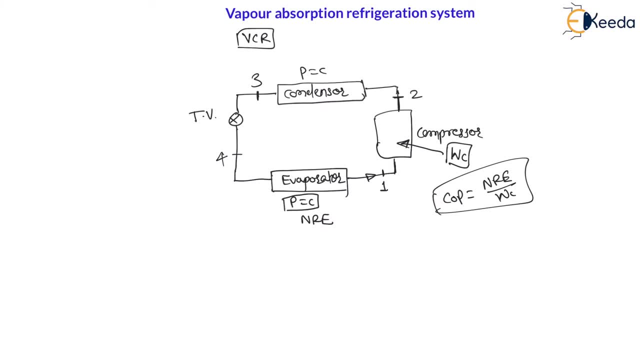 Then compressor. Compressor is a work consuming device And the COP is nothing but net refrigerating effect, That is evaporator load. Here we can say: this COP is nothing but evaporator heat divided by work of compressor. Right. 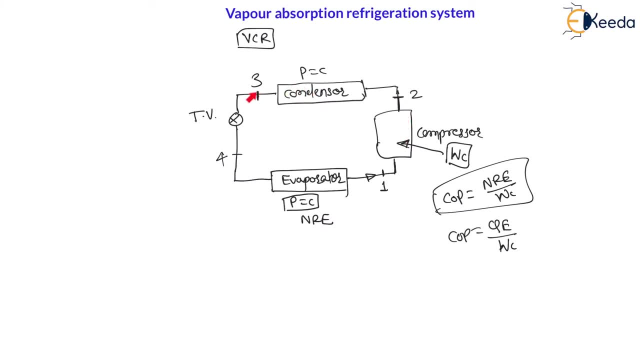 And then, after compression, there is a condenser, And after condenser there is a throttle valve. Now, my dear students, in case of vapor absorption refrigeration system, let us understand here vapor absorption refrigeration system. In case of vapor absorption refrigeration system, let us understand here vapor absorption refrigeration system. 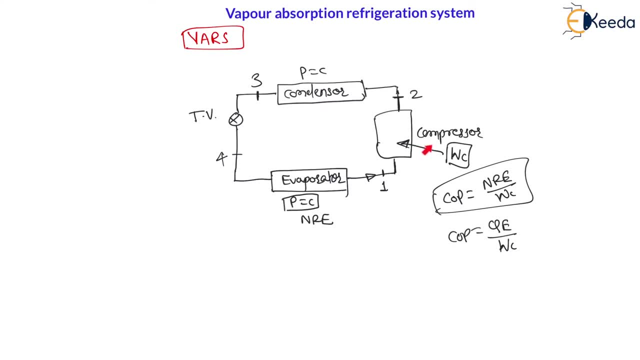 In case of vapor absorption refrigeration system, the compressor of VCR cycle is replaced by absorber, pump and generator Right And other 3 devices will remain same. Therefore here we can say: the evaporator will remain same, then condenser will remain same and throttle valve will remain same. 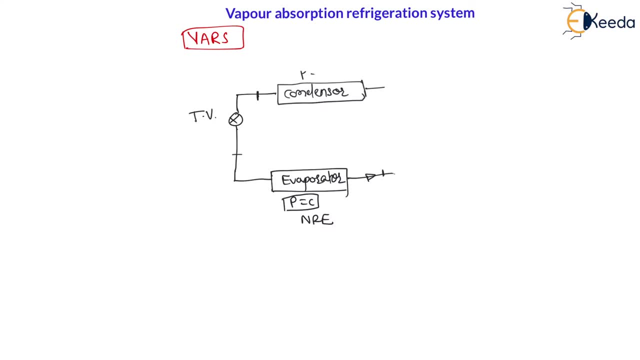 Right, But only here. compressor is replaced with the help of absorber valve: Absorber first, there will be a absorber Here, there will be a absorber Right. Then, after absorption, it is pumped, There will be a pump. 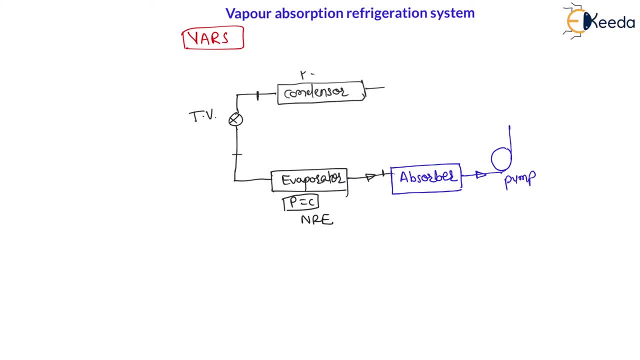 There will be a pump Right And after pumping, there will be a generator. There will be a generator. There will be a generator Right. students, in generator there is always, the generator is always having analyzer. Now I will explain you the purpose of this analyzer: The generator is always having analyzer, Analyzer. 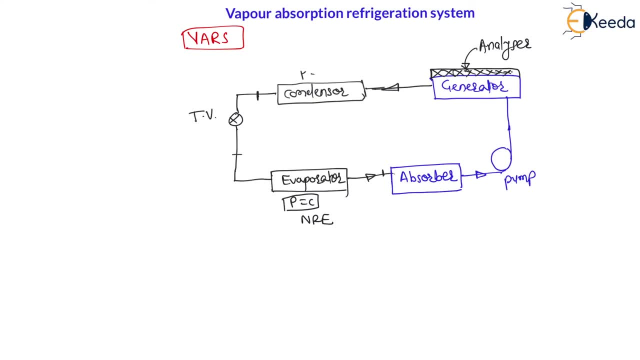 right, and from generator it will go to the condenser, right. So, my dear students, what is the cycle Here? after the evaporation, there is a absorber, then there is a pump, then there is a generator, then condenser and throttle valve. This will be the vapor absorption refrigeration. 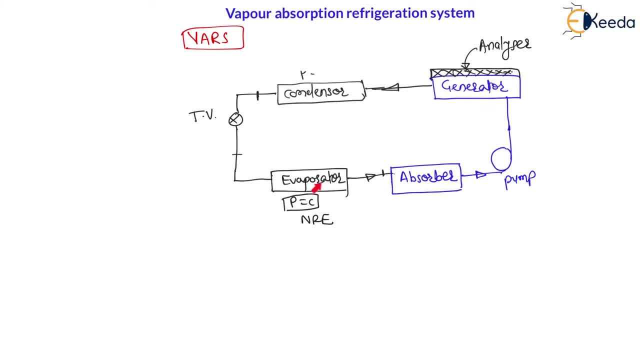 cycle Now, let us understand the meaning of each and every device and why the devices are required. Let us understand these things Now. my dear students, here the COP of the cycle. let me tell you first: COP of the cycle Now, COP is nothing but net refrigerating effect. 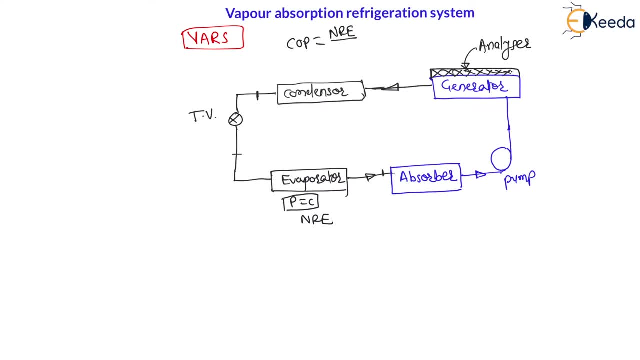 you have a work of compressor in case of VCR cycle. But VCR cycle was work operated and here this vapor absorption refrigeration cycle is working. So here the vapor absorption refrigeration system is heat operated Means in generator. there will be a heat right In evaporator. 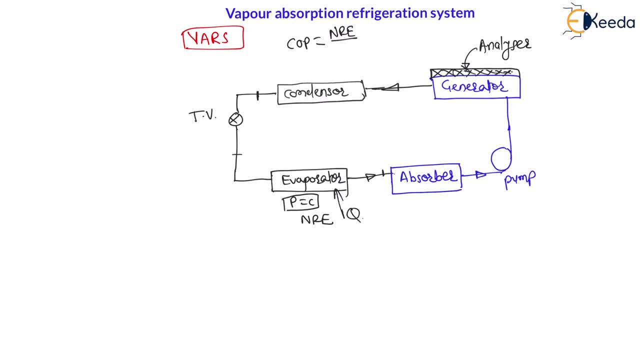 there will be a heat of evaporator. there will be a heat of evaporator and in generator there will be a heat of generator And therefore this COP is nothing but net refrigerating effect from the evaporator divided by heat of generator, Which is nothing but heat of. 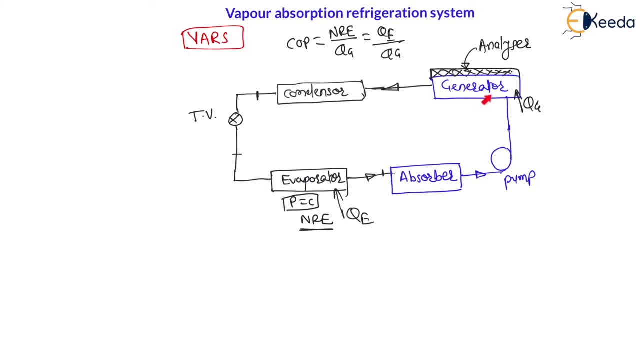 evaporator divided by heat of generator. right, Because in case of compressor, here generator will come. Now, my dear students, let us understand this first: vapor absorption. refrigeration cycle first. Let us understand the devices. Now, my dear students, in case of VCR cycle, refrigerant was used, But here, as there is a evaporator, 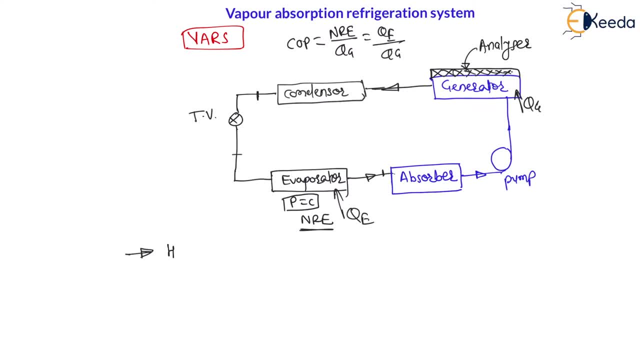 as well as absorber. here refrigerant and absorbent work together. Here we can say: refrigerant, refrigerant and absorbent and absorbent work together. case of vapor absorption refrigeration system: refrigerant and absorbent work together. right now refrigerants are used like here. let us say, for example, we have ammonia, that is NH3 ammonia. 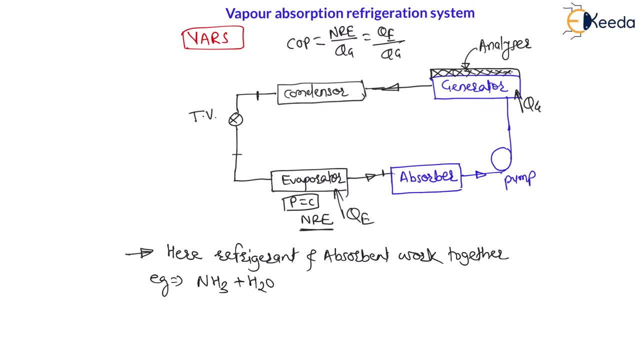 is NH3 plus water. right, in case of ammonia and water, it is also called aqua- ammonia. it is also called aqua- ammonia. aqua means water and ammonia, NH3 means ammonia. right now, my dear students, in case of this aqua- ammonia, the NH3 acts as a refrigerant. ammonia acts as a refrigerant. 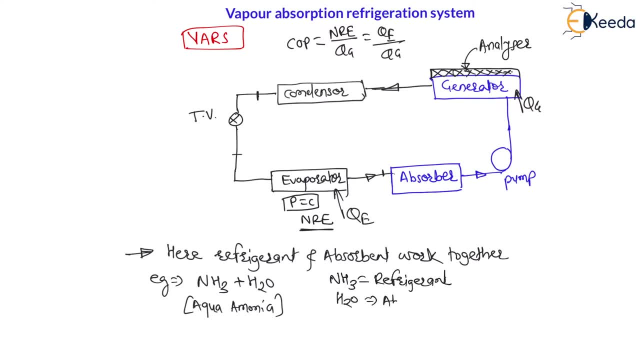 and water acts as a absorber. water acts as a absorbent right and the system is called aqua ammonia system. right again, my dear students, we have water and ammonia right and water acts as a absorber right and the system is called one more refrigerant and absorbent right. we have one more refrigerant and absorbent such 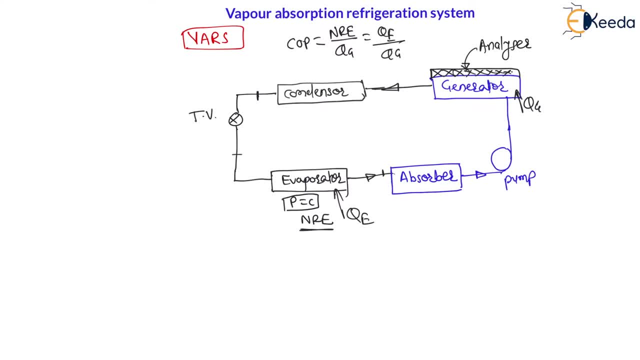 as lithium bromide and water. for example, lithium bromide, LIBR and water and water. right and my dear students, in this case, this lithium bromide acts as a absorbent, acts as a absorbent and water acts as a refrigerant. water acts as a refrigerant. right now, my dear students, 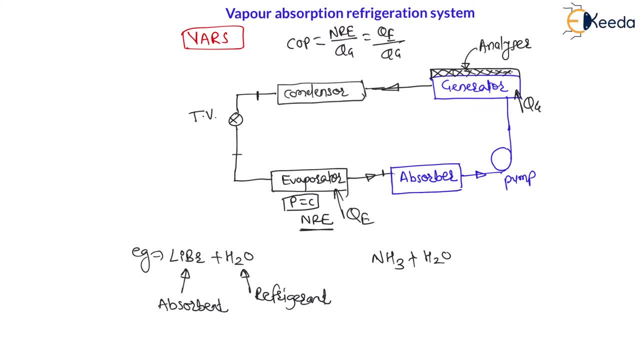 and already we have seen in ammonia water, in NH3 and H2O. ammonia acts as a refrigerant and water acts as a absorbent right. water is absorbent and ammonia is a refrigerant if it is NH3 plus water and if it is lithium bromide plus water, then lithium bromide acts. 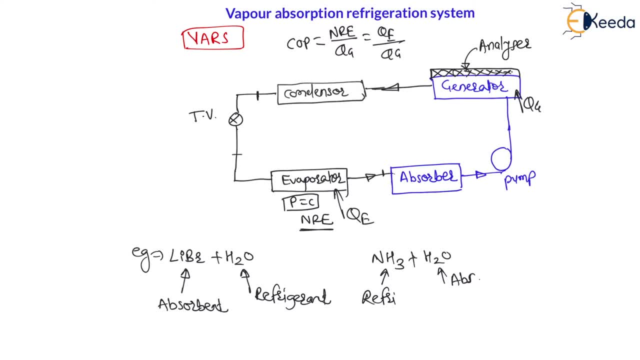 as a absorbent and water acts as a refrigerant. Okay, Let us say: through this cycle, aqua ammonia is a refrigerant. let us say: through this cycle, myosin is aqua ammonia. right, therefore, cycle here I am assuming for ammonia, that is NH3. 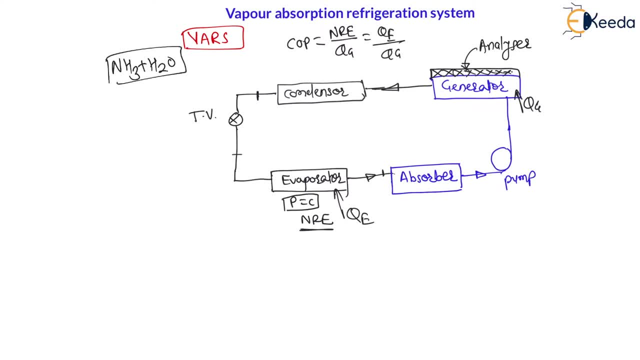 plus water, that is H2O. now ammonia is a refrigerant. here, ammonia is a refrigerant and water is a absorbent. therefore, my dear students, here in evaporator there will be a refrigerant. in evaporator there is a refrigerant, that is, there is a ammonia. 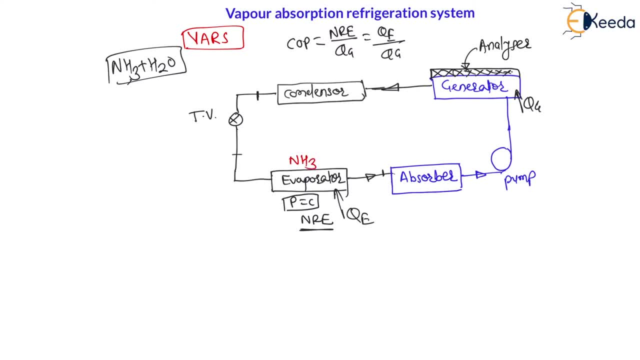 NH3 will be in evaporator and, my dear students, the water will be available in bulk in absorbent, right in absorber. therefore, in absorber there will be a weak solution of in absorber, there will be a weak solution of ammonia and water. Now, the meaning of weak solution of ammonia and water means weak solution of ammonia, means 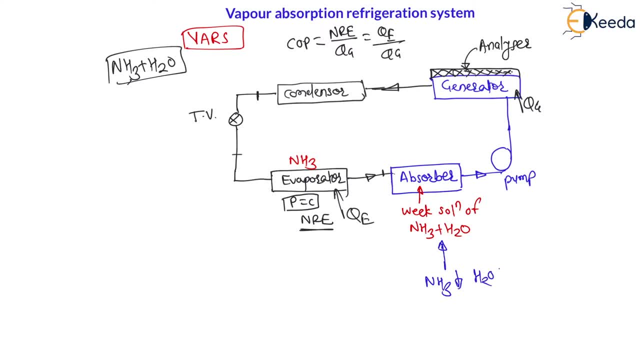 here. ammonia is available very less, But water available is very high. availability of water is very high as compared to availability of ammonia. right therefore there is a mixture of very less quantity of ammonia and high quantity of water. therefore it is called weak solution of aqua ammonia. that is weak solution. 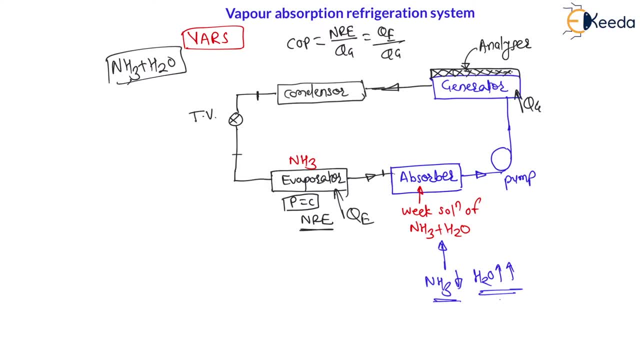 of NH3 plus H2O. right, and my dear students, let us understand here: the water in the absorbent, the water in the absorber absorbs the water. Okay, It absorbs the heat from ammonia. right, therefore, here we can say: in evaporator there is only. 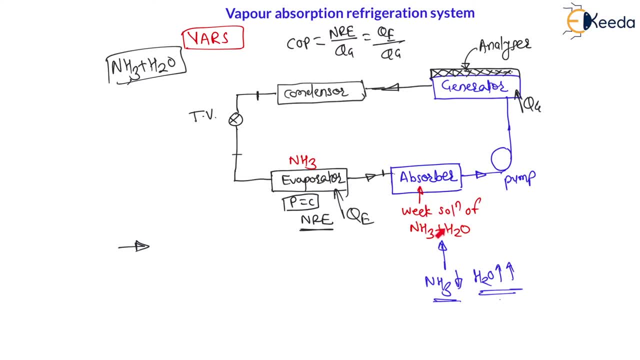 ammonia and in absorber there is a weak solution of ammonia and water and water in the absorber absorbs ammonia from the evaporator right, absorbs ammonia from the evaporator and becomes a strong solution of ammonia water right Now, therefore, we can say the H2O in evaporate absorber. 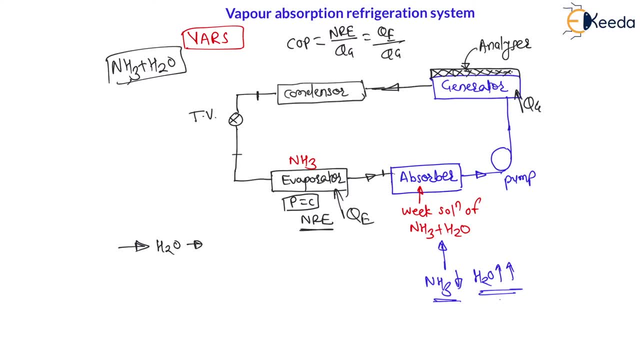 Okay, Now we can say: the H2O in evaporator. Okay, Now we can say: the H2O in absorber absorbs NH3, ammonia, from the evaporator and during this process, lot of heat is absorbed here. lot of heat, we can say lot of heat absorbed. 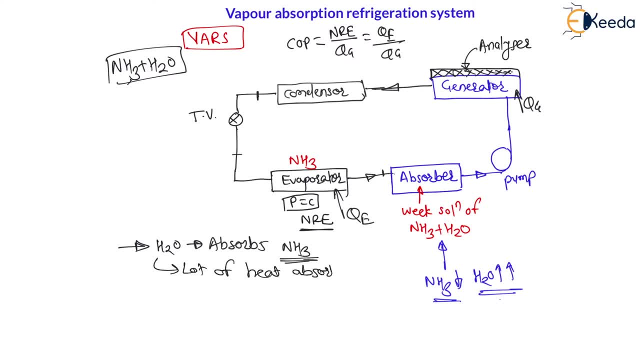 absorbed from ammonia. right Now, my dear students, as water is absorbing ammonia. therefore this NH3 plus H2O, here the, the quantity of NH3 is increasing and water is remaining same. Therefore, as quantity of NH3, that is, ammonia, is increasing. 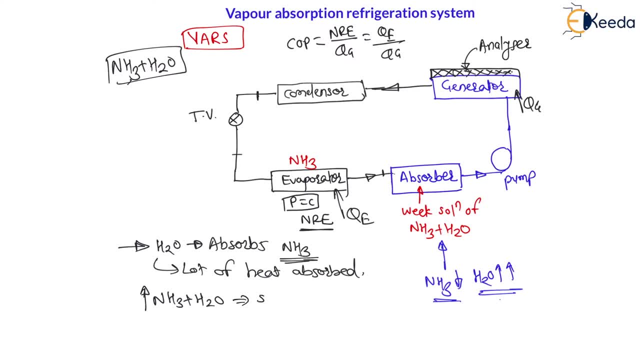 therefore, the solution becomes strong solution of NH3.. Now, this is a strong solution. We can say this is a strong solution of ammonia and water. Now, my dear students, once this strong solution is formed in absorber, that is, once the water from absorber absorbs ammonia from the evaporator, 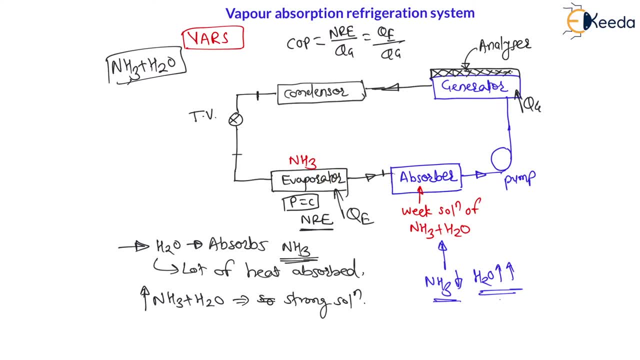 during this absorption, lot of heat is absorbed by the water and this strong solution of ammonia and water is pumped through the pump to the generator. Now, here there is a water and ammonia in liquid form. Now this ammonia water. that is strong solution of ammonia and water. 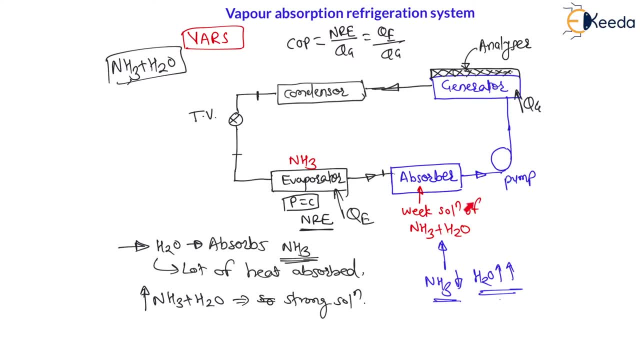 is pumped through the pump to the generator. Now, the purpose of pump is to pump absorber pressure to the generator pressure. Right Now, my dear students, let us understand the purpose of generator. Now, my dear students, as the strong solution of ammonia and water goes to the generator, 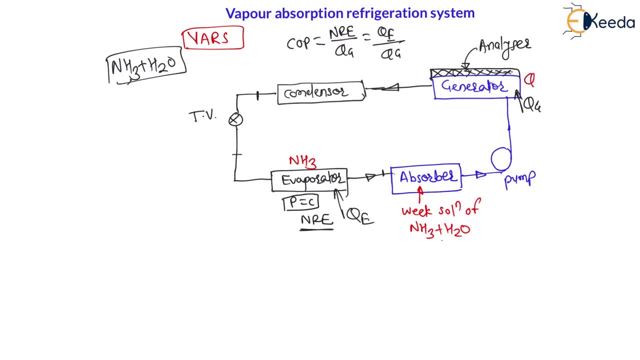 this generator will supply generator heat, That is, heat of generator is supplied to this ammonia plus water mixture and this generator will convert this liquid ammonia water, NH3 plus H2O, into vapor Vapor: ammonia plus water Right Now. so, my dear students, 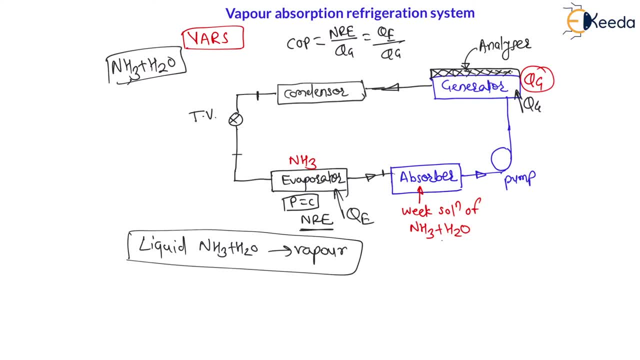 the purpose of generator is to supply heat of generator so that this liquid NH3 plus water will convert into vapor. Right, Because, my dear students, here, for condenser vapor is required, Because in condenser, if liquid particle goes, then there will be a 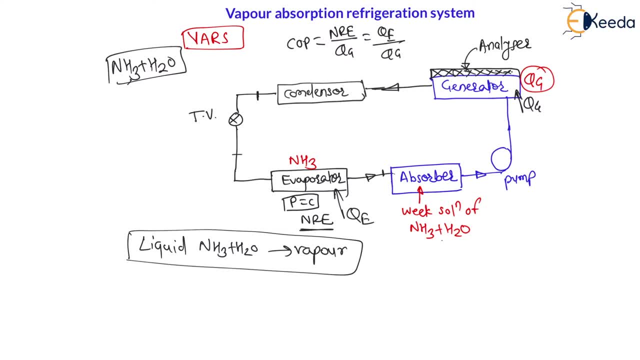 losses will increase and there will be a more problem for the condenser. Therefore here, the purpose of generator is to convert this liquid ammonia water into the vapor before passing to the generator. But, my dear students, in the generator 100% conversion of liquid ammonia and water into vapor is not possible. 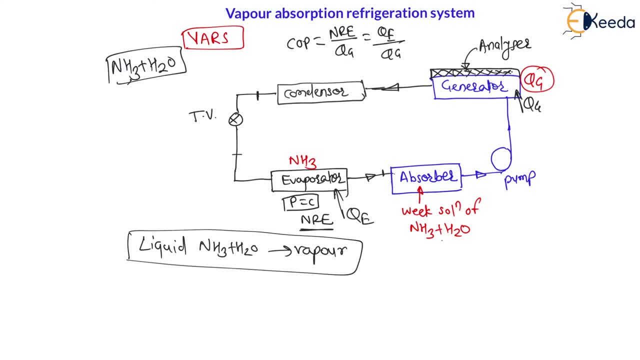 So again there is some quantity of- we can say there is some quantity of- ammonia plus water in liquid form And this is now weak solution. We can say this is a weak solution because lot of converted into vapor and going gone into the condenser. 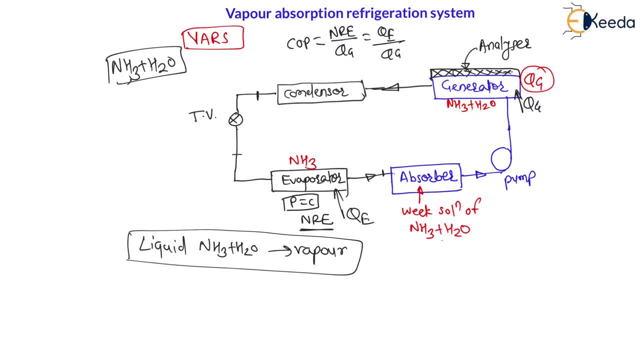 Right Now, whatever may be, the liquid portion is remaining now here, there will be a pressure reducing wall is used. The pressure reducing wall is used. The arrangement is like this. I will show you here: There will be a pressure reducing wall. 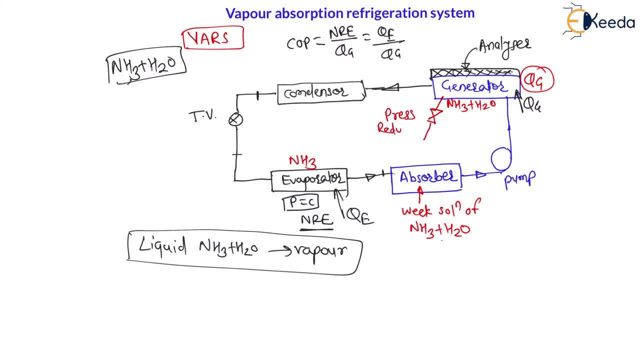 This is called pressure reducing wall. Now, my dear students, we will use pressure reducing wall. Now, this pressure reducing wall, what will do this? This will supply this liquid ammonia plus water back to the absorber. My dear students, now, in generator, whatever may be, the vapor is generated. 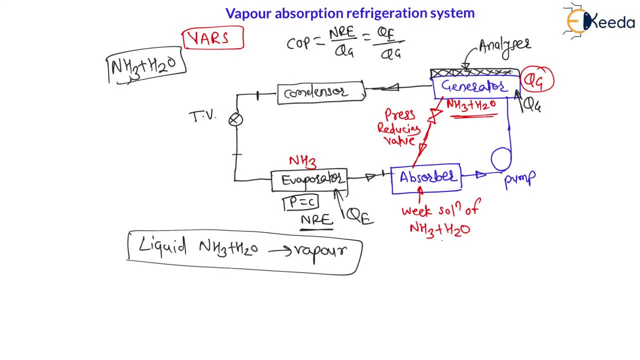 vapor of ammonia and water is generated. This vapor goes into the condenser and the liquid ammonia water, which is the weak solution, will go back through the pressure reducing wall to the absorber. back Now, my dear students here, the purpose of analyzer. 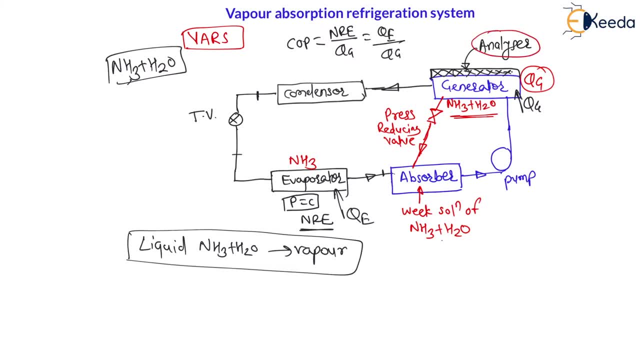 Let us understand the purpose of analyzer. The purpose of analyzer is same, That is, the analyzer will ensure that only vapor is entering into the condenser. right means here we can say to the condenser, only vapor is passing and liquid ammonia will go through the pressure reducing wall back to the absorber. 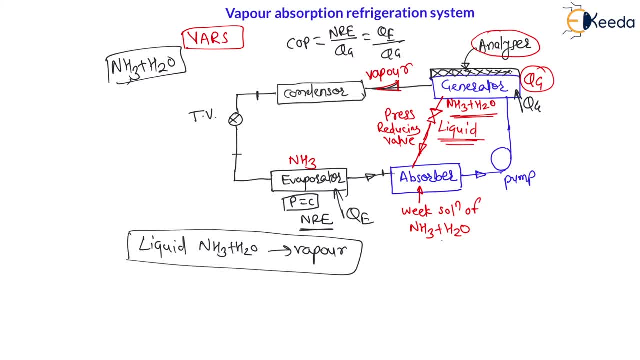 The purpose of this analyzer is to ensure that only vapor will go to the condenser and liquid will go to the absorber. This is the only purpose of this analyzer. right Now, let us understand here COP of this cycle. COP is nothing but coefficient of performance in the number. 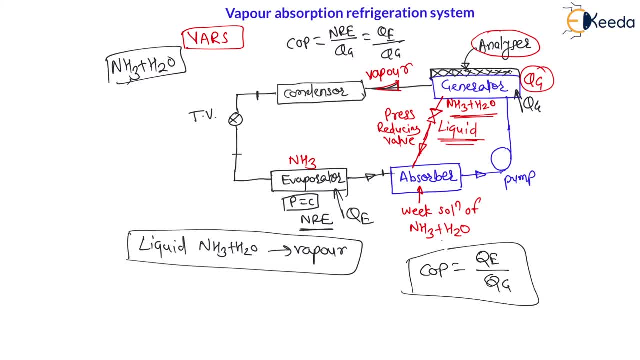 Heat of evaporator divided by heat of generator. right Now, here our target is to find this COP, So let us draw here block diagram of this vapor absorption refrigeration system. Now, once the vapor passes through the condenser, in condenser again, it will convert this vapor into liquid state, right? 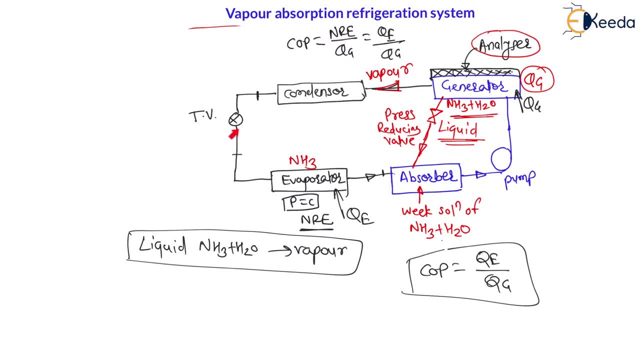 And again in throttle wall there will be throttling. That is isenthalpic process. And again through the throttling it passes through the evaporator Means. rest operations are exactly similar to VCR cycle, That is, vapor is passing through the condenser. 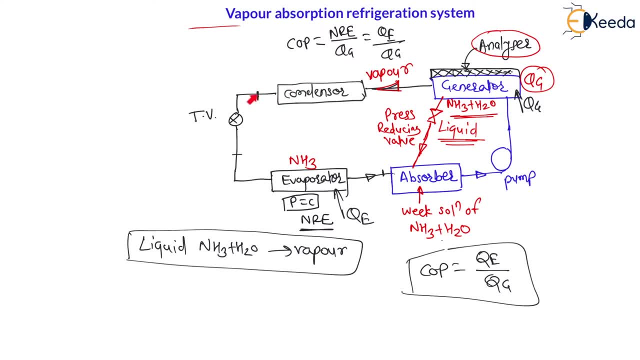 At the end of condenser there is always saturated liquid state. Now this saturated liquid state is throttled in the throttle wall, where enthalpy remains constant, but entropy increases, quality increases and temperature drops right. And from throttle wall again, the mixture passes through evaporator. 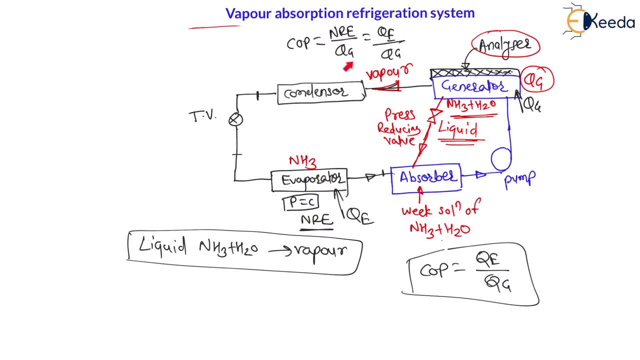 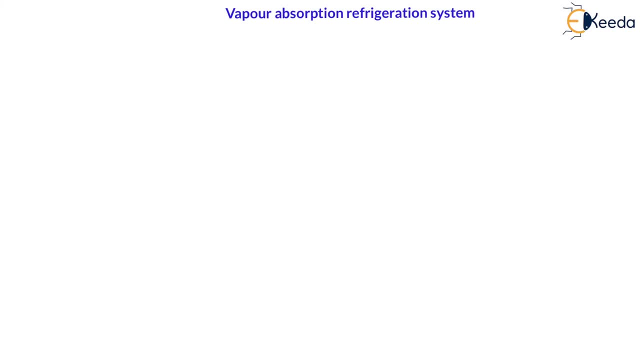 where there will be a net refrigerating effect. And again the cycle will continue. Again, the cycle will continue. Now let us understand the block diagram of this vapor absorption refrigeration system and find COP. Now, my dear students, in block diagram, if I see, we have a generator. 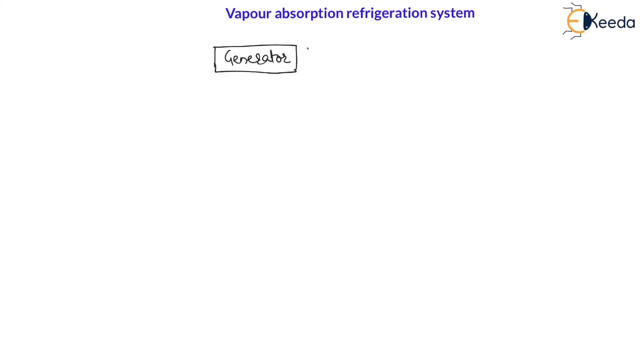 We have a generator at temperature of generator. Let us say Tg is generator temperature, Generator temperature right Now from generator. the heat of generator is going into the heat of generator is going into condenser: right From generator there is a condenser. 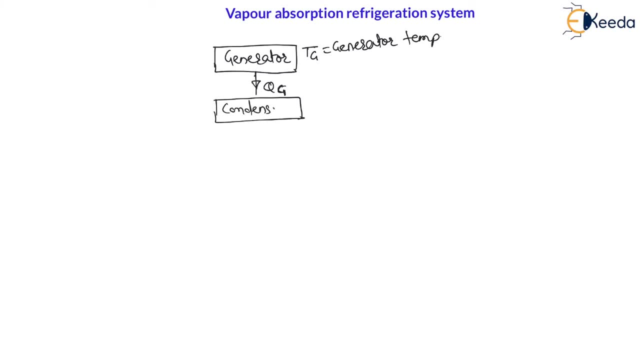 There will be a condenser And this condenser will be at condenser temperature. Temperature of condenser, Temperature of condenser, is Tc right And, my dear students, this condenser is rejecting heat to the surrounding right. Therefore, this heat of condenser- we can say the heat of condenser- is going into the surrounding. 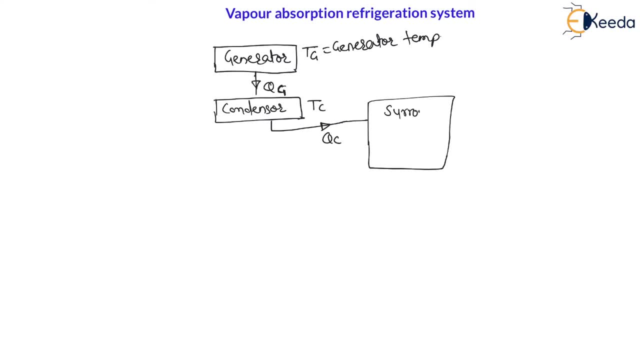 Let us say there is a surrounding, There is a surrounding And surrounding, let us say at temperature T0.. Temperature of surrounding is considered as T0,. right Now this is one cycle, That is, heat of generator is going into condenser. 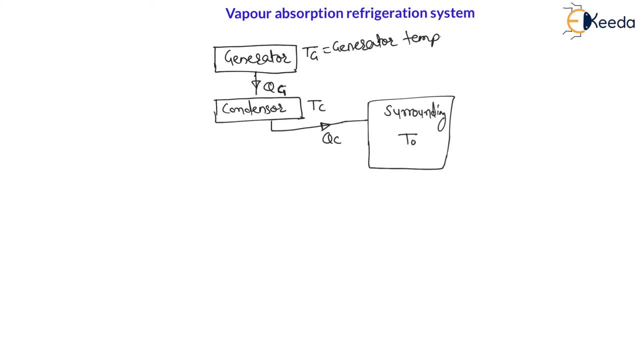 Heat of condenser is going into surrounding And surrounding is at T0.. At temperature T0.. Again there is a evaporator, Again there is a evaporator. right Now, this evaporator is at evaporator temperature right. 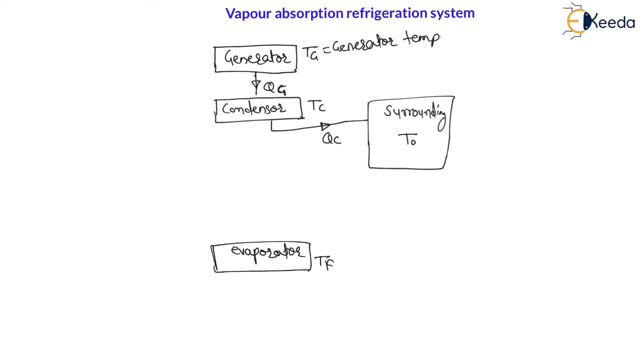 This evaporator will be at temperature of evaporator. Te is evaporator temperature, Evaporator temperature. Now, my dear students, from evaporator, the heat of evaporator, which is nothing but net refrigerating effect, is going into the absorber. 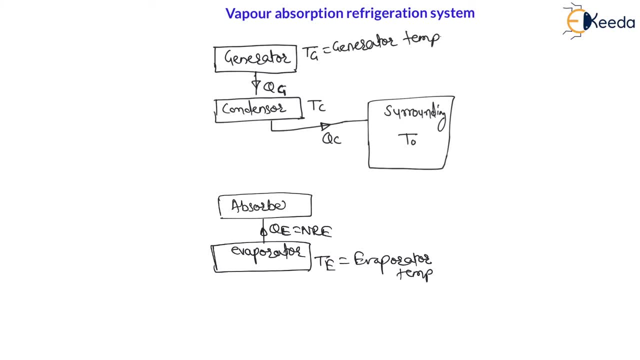 There is a absorber right. There is a absorber at temperature of absorber right Now. there is no significance of temperature of condenser and temperature of absorber. Now again, in this absorber the water will absorb heat from the ammonia. 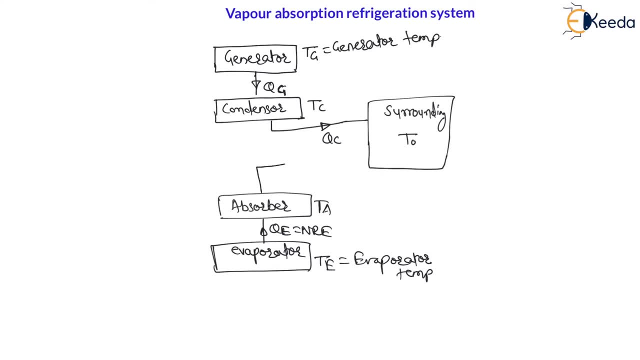 And this heat is rejected to the again. surrounding Water will absorb lot of heat from the ammonia And this heat of absorber is again rejected to the surrounding only Means heat of condenser as well as heat of absorber. 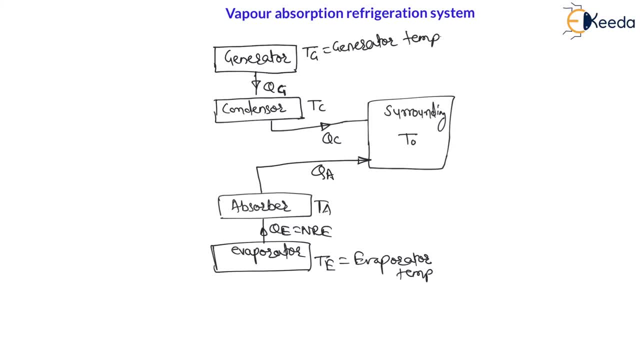 As well as heat of absorber is rejected to the surrounding Right And the net refrigerating effect is obtained in evaporator Right, And here the COP of cycle. COP of cycle is nothing but heat of evaporator divided by heat of generator. 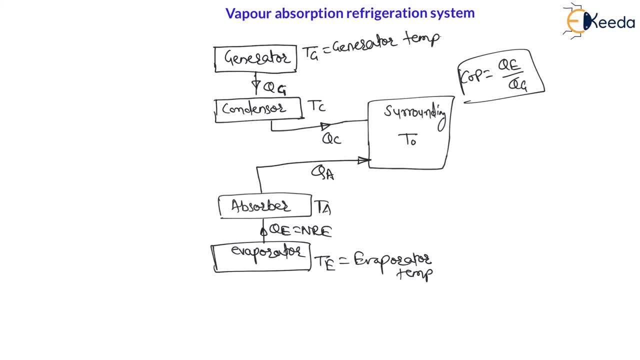 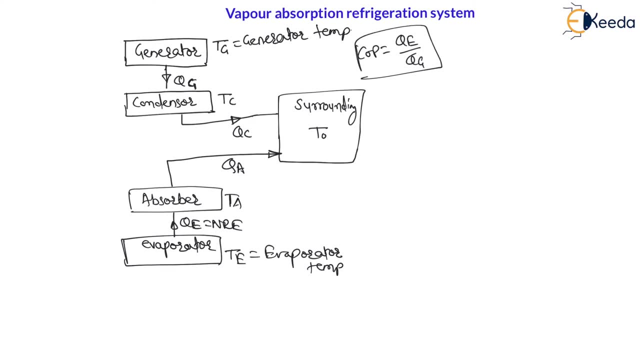 Right. So in this system, let us find this COP. Now, my dear students, for this system, let us apply first law of thermodynamics. For this system, apply first law of thermodynamics As per first law of thermodynamics. 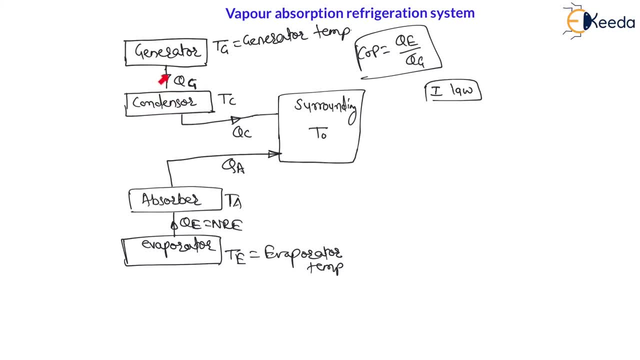 we can say: whatever may be the energy entering into the system, that is, energy entering into system is Qg and Qe. Therefore, energy entering that is Qg plus Qe must be equal to energy leaving. Now, energy leaving is heat of condenser and absorber heat. 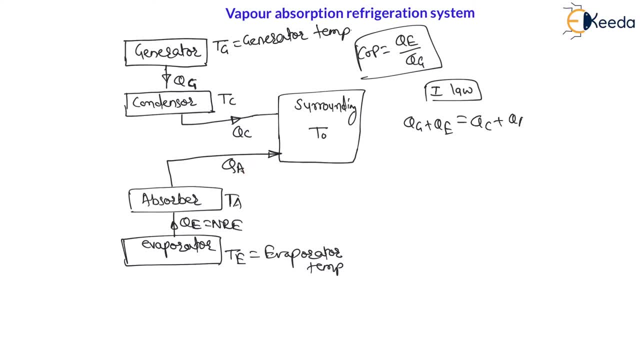 Therefore, is equal to Qc plus Qa. This is called first law of thermodynamics. Let us say this is our first equation. Energy entering into the system, that is, Qg plus Qe, is equal to energy leaving the system to the surrounding. 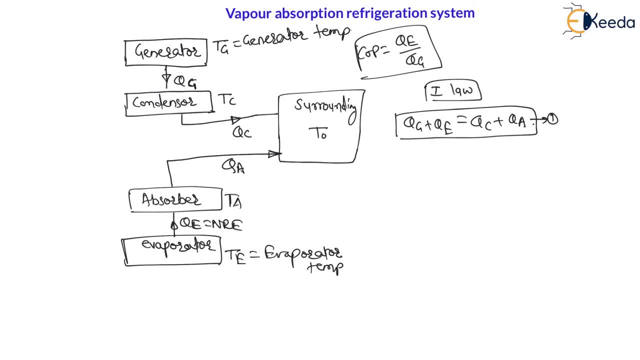 That is Qc plus Qa. Right Now again apply second law of thermodynamics. Second law of thermodynamics, That is Clausius inequality for reversible cycle. Now for reversible cycle. Here my assumption is: this cycle is reversible cycle. 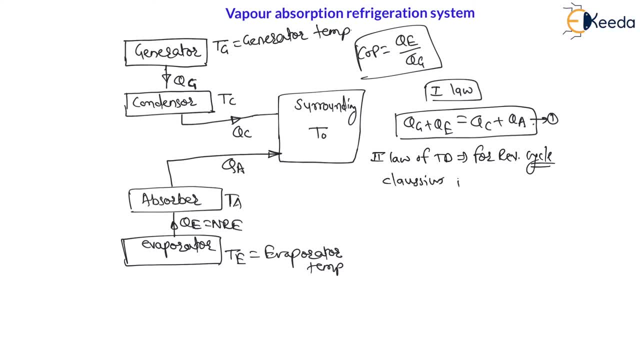 Apply Clausius inequality Now. as per Clausius inequality, the cyclic integral of dq by t is equal to zero for reversible cycle. For reversible cycle, cyclic integral of dq by t is equal to zero. Right, This is called Clausius inequality. 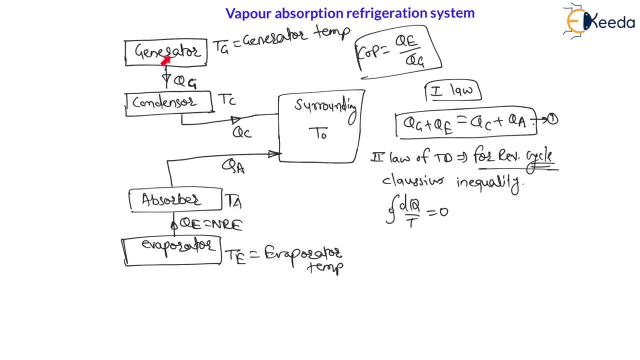 Now let us observe here Now, if I consider generator, for this generator, Qg- amount of heat is rejected from the generator. Therefore, for this generator, Qg is negative heat. Heat rejected from the system is negative heat And it is at temperature of generator that is Tg. 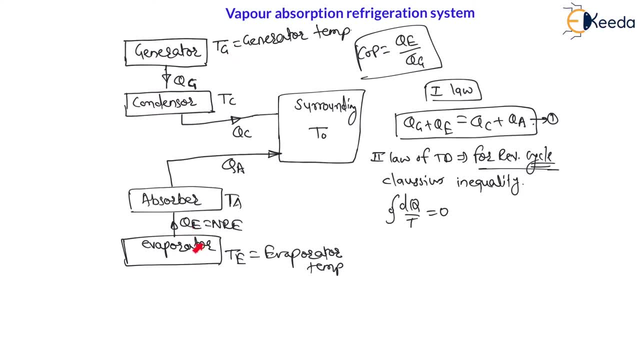 Again for evaporator. Qe amount of heat is rejected from the evaporator at temperature of evaporator. Therefore this heat of evaporator is negative heat for this evaporator And in a surrounding Qc and Qa amount of heat is entering. 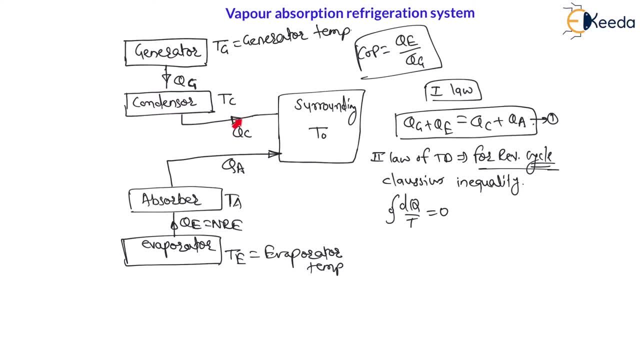 That is therefore for this surrounding at temperature T0, this Qc and Qa is a positive heat. Whenever heat is given to the system, it is a positive heat. Whenever heat is rejected from the system, it is a negative heat. 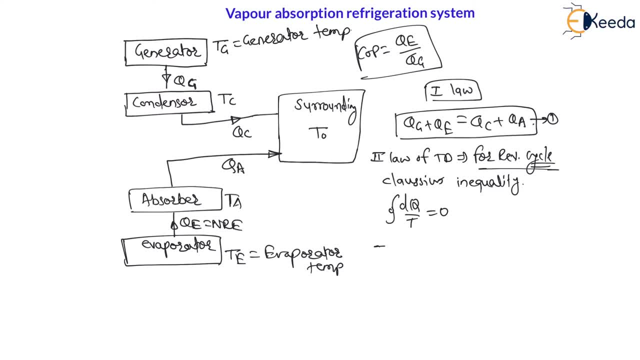 Therefore here cyclic integral of dq by t can be written as: minus Qg at temperature Tg, minus Qe at temperature Te, plus Qc at temperature T0, plus Qa at temperature T0 is equal to zero. This is called Clausius inequality. 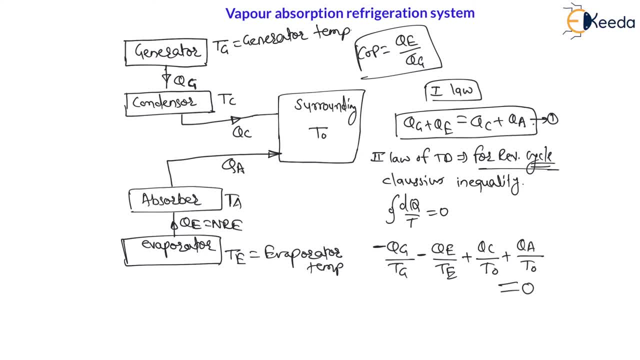 Right. So, my dear students, let us simplify this Clausius inequality Here. I am removing block diagram so that we will get sufficient space for the simplification of this Clausius inequality Right Now, my dear students. so from here. 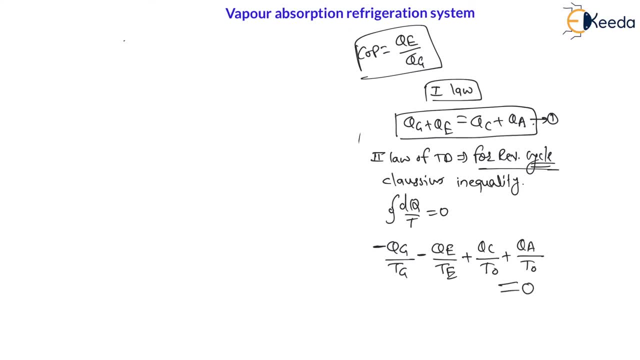 consider positive term on one side and negative term on the other side, Then these negative terms will become positive if I pass them to the right side. Therefore, we can say Qc divided by Te0 plus Qa divided by Te0,. 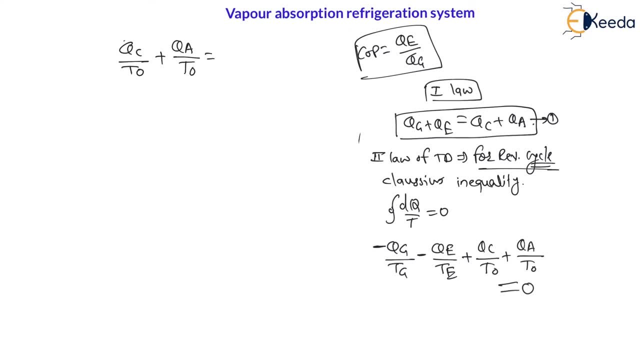 Qc divided by Te0 plus Qa divided by Te0, is equal to Qg divided by Tg plus Qe divided by Te0,. evaporator temperature: Right And always. my dear students, remember one thing: the generator temperature is more as compared to surrounding temperature, is more as compared to evaporator temperature. 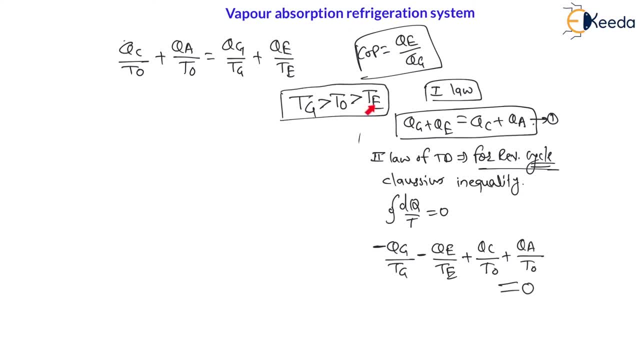 Always this is the case. The lowest temperature is for evaporator and the maximum temperature is for generator, and surrounding temperature is in between, Because net refrigerating effect is obtained in evaporator. Therefore, there must be a lowest temperature, And it is obtained with the help of generator. 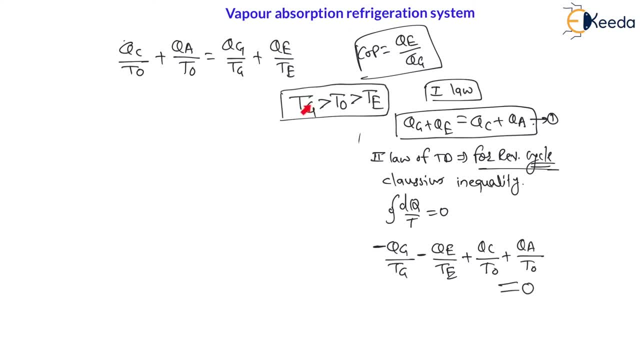 Therefore, in generator there is a maximum temperature Right Now. let us simplify again here, My dear students. here there is a common denominator. Therefore, this Qc plus Qa, Qc plus Qa from equation number one: 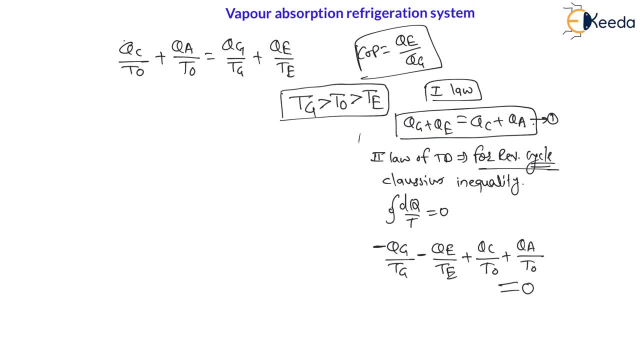 can we write it is Qg plus Qe. Therefore, this Qc plus Qa divided by Te0 is equal to Qg divided by Te0, Qg divided by Tg plus Qe divided by Te. Therefore, this Qc plus Qa can be written as Qg plus Qe. 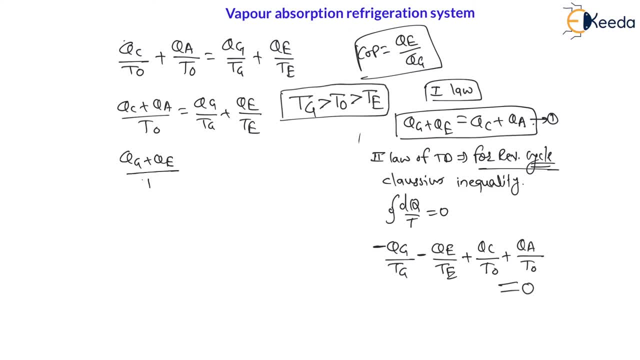 Therefore, Qg plus Qe divided by Te0 is equal to Qg divided by Tg plus Qe divided by Te. Right Again, let us simplify this Now here. I will remove this So that we will get sufficient space for the complete solution. 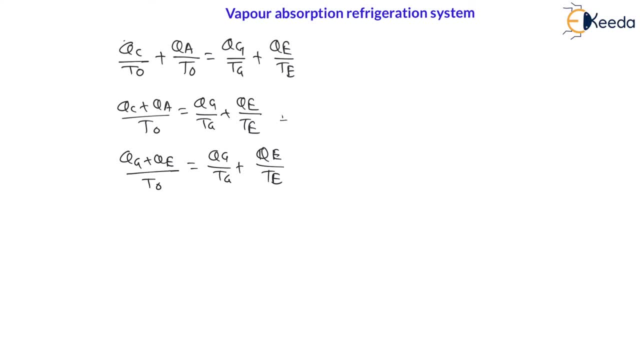 Now let us simplify again. Now consider Qg terms on one side and Qe terms on one side. Therefore here Qg divided by Te0 minus Qg divided by Tg is equal to Qe divided by Te minus Qe divided by Te0. 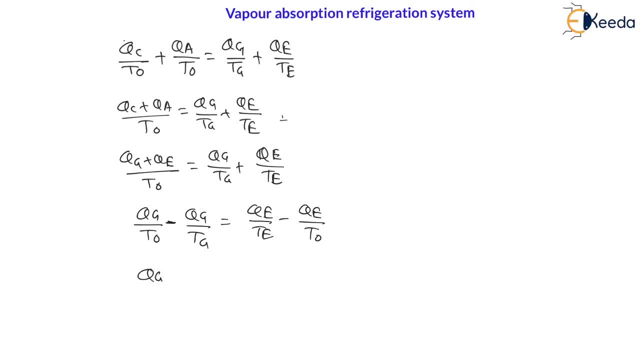 Right Again. consider Qg common. Therefore Qg in bracket one upon Te0 minus one upon Tg is equal to consider Qe common from the right side, Therefore Qg common from the left side. so 1 upon Tg minus 1 upon Te0 minus 1 upon Te0. 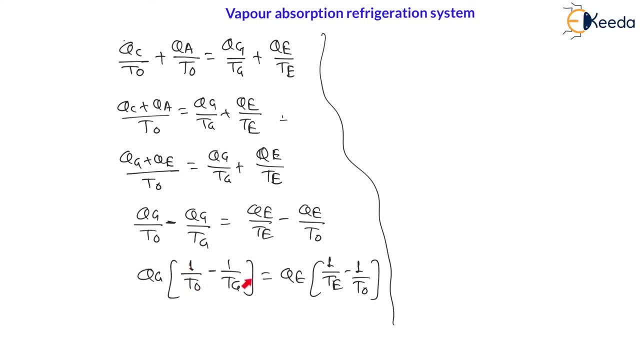 This is very simple, my dear students. Here I am only simplifying the equation, that you must be able to simplify such type of equations. Now, here again, cross multiplication, Simplify again. Therefore, we can say: Qg into Tg minus Te0, divided by Te0Tg is equal to 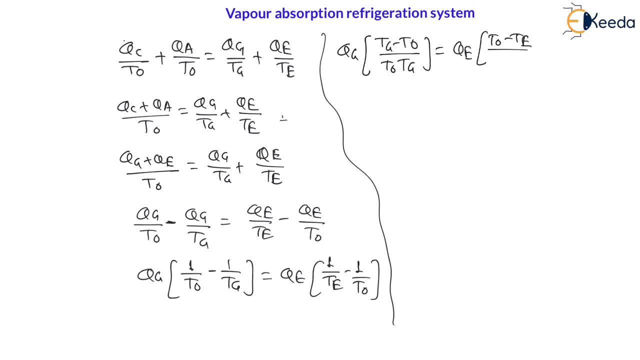 Qe into bracket T0 minus Teprather Р g. tg divided by Te0Tg is equal to minus TE divided by T0 TE. This equation we will get. Now let us find QE divided by QG. Therefore, this QG I will take on right side and this ratio I will take on left side. Now from: 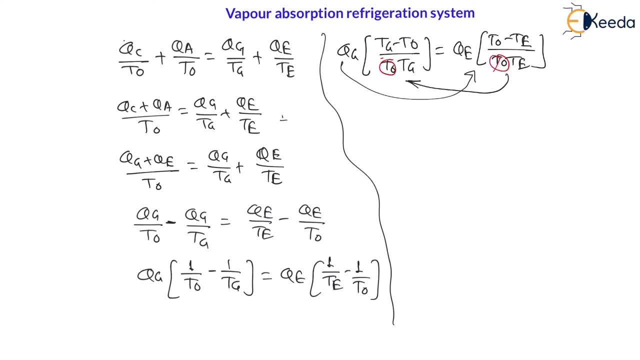 both side. can I say T0, T0 will get cancelled, Right. Therefore, my dear students, we will get TG minus T0 divided by TG into TE. divided by T0 minus TE is equal to heat of evaporator divided by heat of generator. And, my dear students, this heat of evaporator divided by heat of generator, 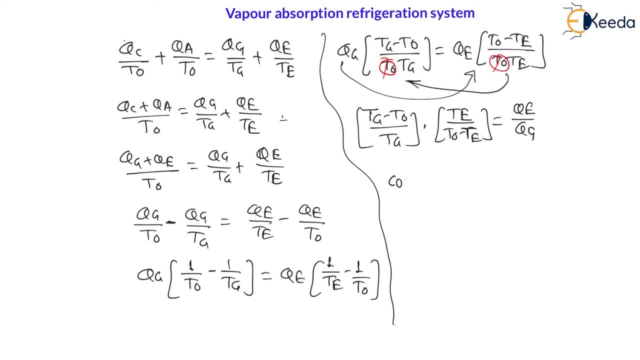 is nothing but COP. Therefore, here we will get COP of cycle for vapor absorption refrigeration system, COP, which is nothing but heat of evaporator divided by heat of generator, and evaporator is at lowest temperature and generator is at highest temperature and surrounding is at intermediate. 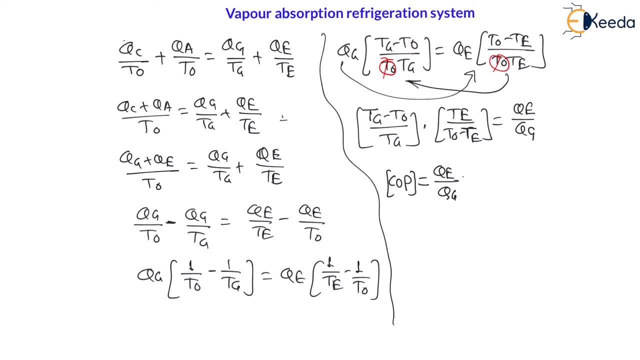 temperature is equal to. this is equal to. we can say here: TG minus T0 divided by TG into TE, divided by T0 minus TE. Right Where TG is generator temperature, T0 is surrounding temperature and TE is evaporator temperature. Right Now, my dear students, 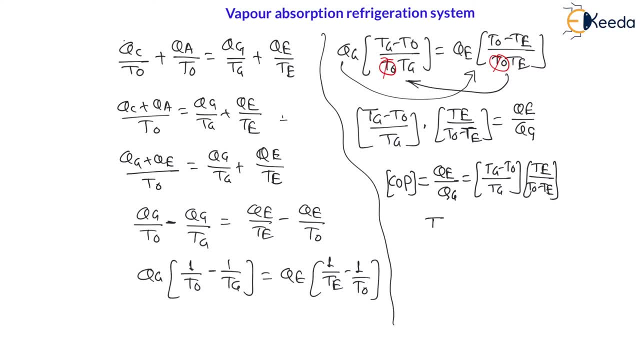 here this formula is very much important And where we have TG is more than T0, is more than TE. Now let us simplify this formula. Here I will explain you one trick to remember this formula. Now, here I will tell you the trick to remember this formula, because sometimes students feel 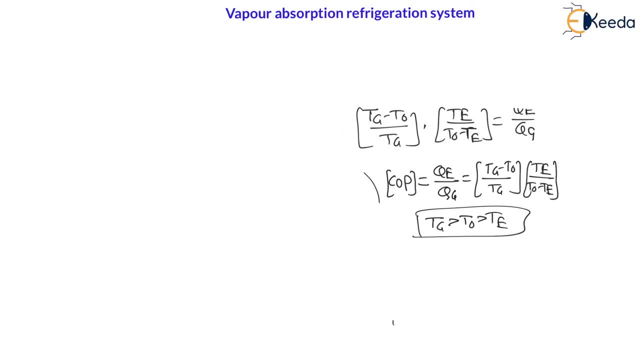 difficulty to remember this formula because in many times in examination they will provide you the condenser temperature also. but condenser temperature is not useful for finding COP of this vapor absorption refrigeration system, Only generated temperature, surrounding temperature and evaporator temperature are required. Now, here I will tell you the short trick to remember this formula. Now, my dear students, 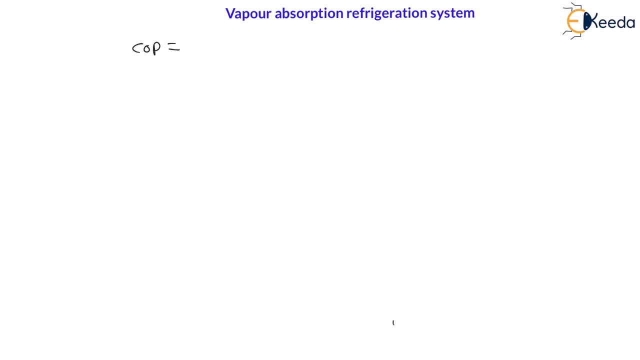 here let us say the COP of this vapor absorption refrigerationThank you for watching this video. If you liked this video, do subscribe to this channel and hit that bell-notified icon button to get potatoes updated. Press that bell icon to get quieter videos. Bye and advancing. 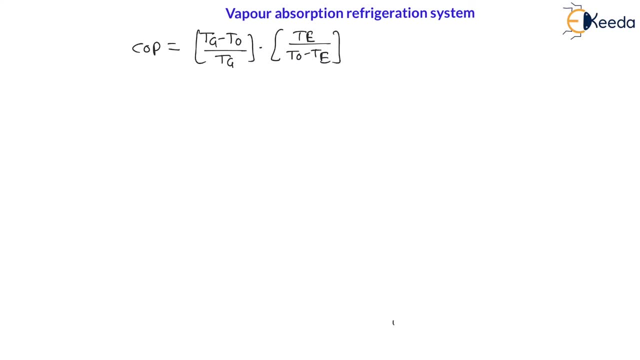 T0 minus Te. right, this is the COP finding formula. now, my dear students, again the formula can be written as is equal to 1 minus, if I divide with Tg separately, 1 minus T0 divided by Tg into Te, divided by T0 minus Te. this will be the formula. now let us say, my dear students, we have. 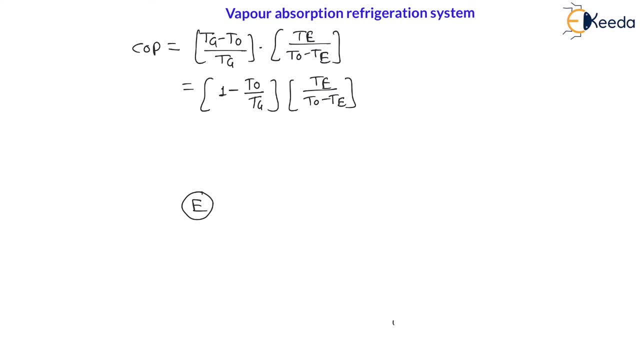 one Carnot engine. let us say we have one Carnot engine operating between the higher temperature, Tg, which is constant, and lower temperature of surrounding T0, which is constant. now the purpose of engine is to absorb heat from the generator. that is higher temperature, qg. amount of heat is. 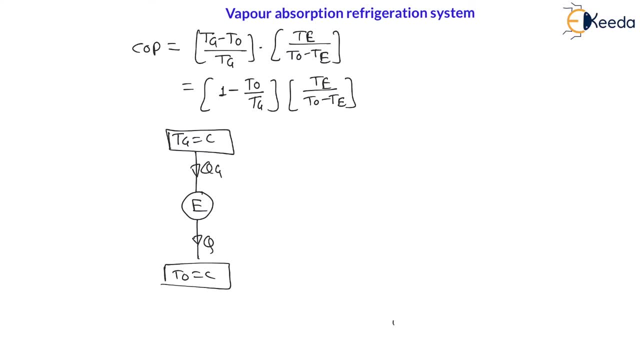 absorbed and reject heat to the surrounding. let reject heat to the surrounding. q amount of heat is rejected to the surrounding, T0 and produce what it will produce: network output. the net output produced is qg minus q right heat from the higher temperature reservoir, minus heat rejected to the surrounding. right now, this is one engine. 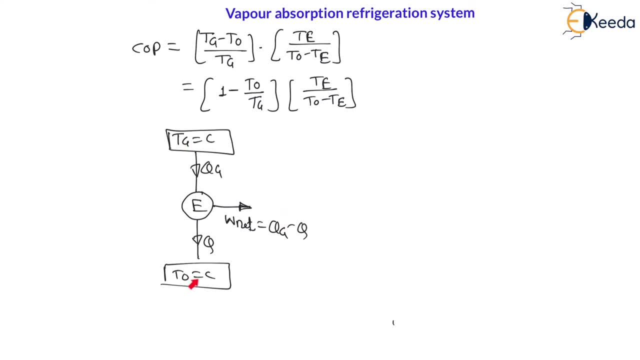 operating between higher temperature Tg and lower temperature T0. now, if it is Carnot engine, the efficiency of this engine is given, as efficiency of this Carnot engine operating between T0 and Tg is nothing but 1 minus lower temperature T0, they have a higher temperature T0. 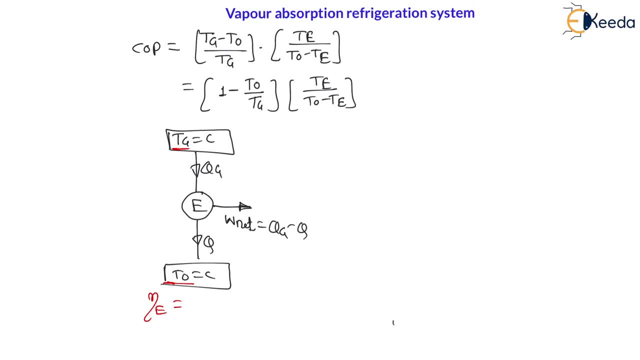 Tg. this formula, we have 1 minus 1, minus lower temperature, divided by higher temperature. this is the efficiency of engine. now, my dear students, whatever may be the work, output from the engine is given to the refrigerator. now, Carnot refrigerator- here I am assuming Carnot refrigerator. let us say: 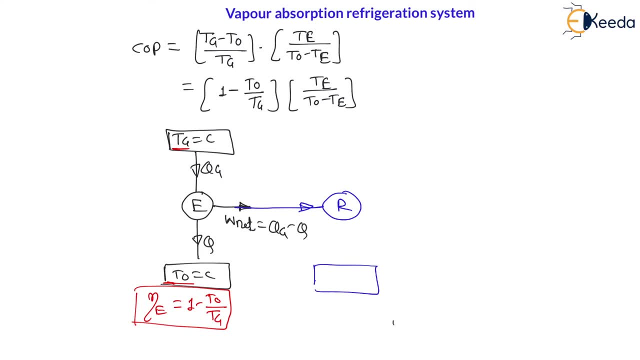 there is a Carnot refrigerator and this refrigerator operates between the lower temperature of evaporator temperature, which is constant, and higher temperature of surrounding temperature, which is again constant. let us say T0 is constant. now the purpose of this Refrigerator is to extract heat from the evaporator, which is visible heat of evaporator, and continuously supply. 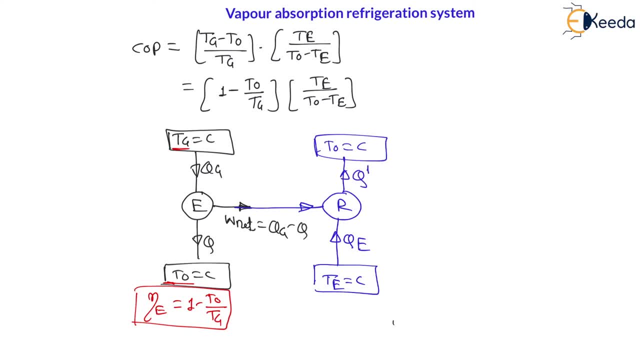 to the surrounding. let us say here: q dash is supplied to the surrounding right. this is the purpose of refrigerator, which will extract heat from the lower temperature reservoir and continuously supply to the higher temperature reservoir by consuming work right. therefore, q dash is supplied to the higher temperature. 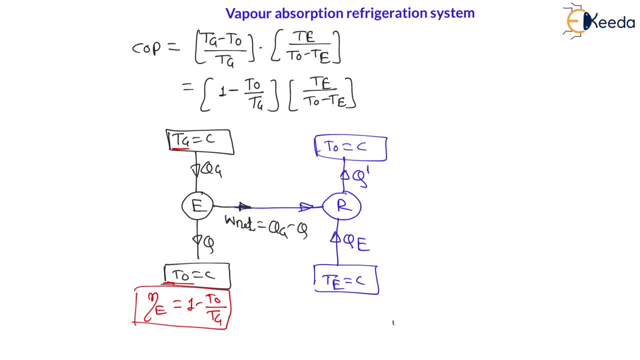 temperature is required. now, my dear students. so here, in previous case, TG is more than T0 and in next case T0 is more than TE. therefore minimum temperature is. so in cycle, we can say: TG is more than T0, is more than TE, and E is for evaporator, O is for surrounding, G is for generator. now, my dear, 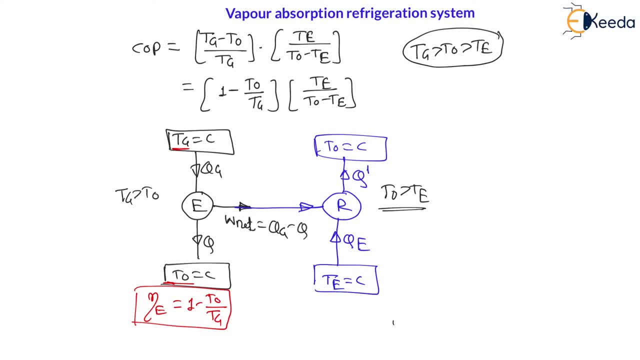 students for this refrigerator. the COP in terms of temperature. COP of this refrigerator is nothing but the lower temperature TE. they have a difference of temperature that is T0 minus TE. this formula to find that is COP of Carnot refrigerator we have already seen in theory lectures. and this formula to find efficiency, already we have seen in theory lectures. 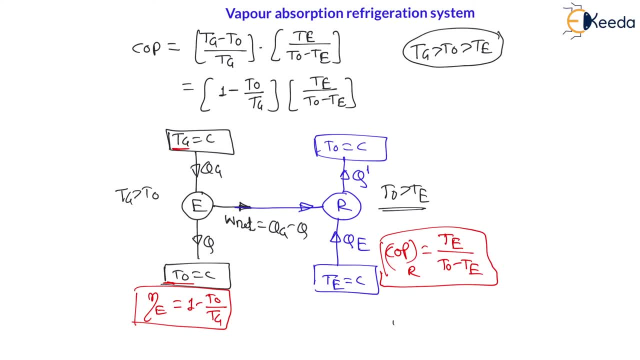 right. so, my dear students, if engine operating between TG and T0 and refrigerator operating between TE and T0 are taken together, then the COP of this cycle is going to be equal to TG of Carnot refrigerator. we have already seen in theory lectures and this COP of vapor absorption refrigeration here, sorry, vapor absorption refrigeration system. 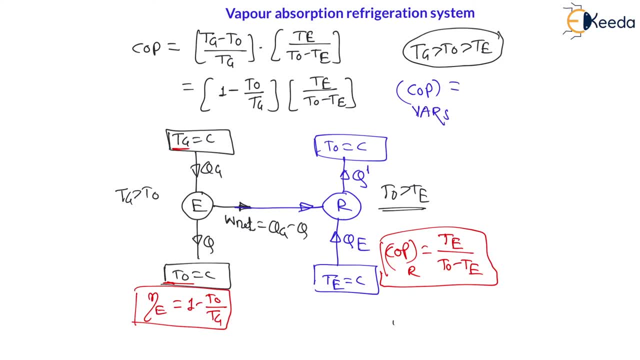 COP of vapor absorption refrigeration system will be equal to. we have just seen 1 minus T0 divided by TG into TE. divided by T0 minus TE, this formula we will get. therefore, COP of vapor absorption refrigeration system will be equal to efficiency of engine. but this engine is 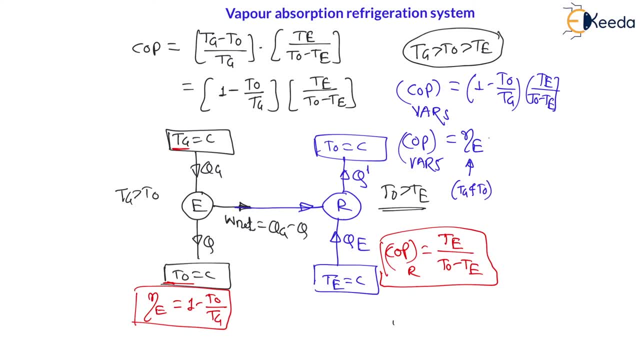 operating between temperature limits TG and T0 into COP of Carnot refrigerator. but this refrigerator is operating between temperature limits of TE and T0, right? this is the short trick to remember the formula, right. so, my dear students, if you are able to remember this directly formula, then no problem. 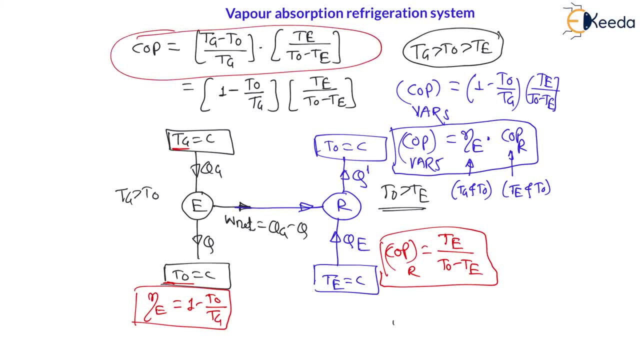 right. if you remember direct this formula then no problem. if you forget, try to remember by this concept, because efficiency of engine and temperature limits are the same. so if you remember this COP of Carnot refrigerator is finding already we have seen in second law of thermodynamics, right. 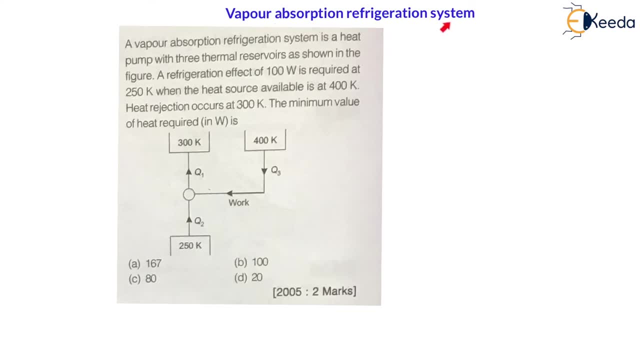 now, my dear students, let us understand this. vapor absorption refrigeration system through a previous year gate numerical. now here. this question was asked in gate 2005 for 2 months now. the question is based on vapor absorption refrigeration system. let us understand the question. a vapor absorption refrigeration system- here var system is one- is a heat pump with three thermal. 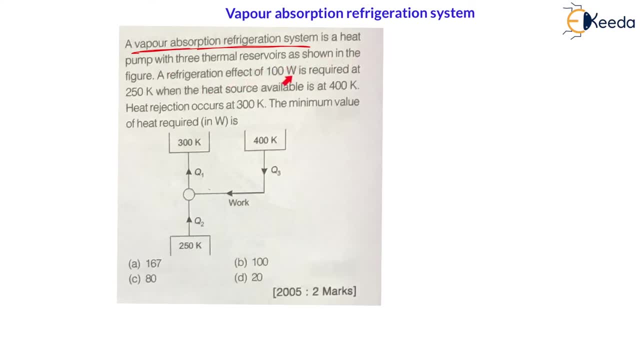 reservoir, as shown in figure. the refrigeration is a heat pump which is a 3-thermal reservoir, as shown in figure. the refrigeration system showed in 2 months. the refrigeration system showed in 2 months. refrigeration effect of 100 Watt is required at 250 Kelvin. now at 250 Kelvin. 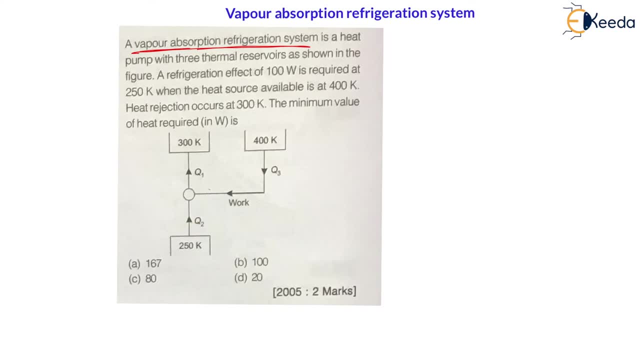 refrigeration effect, that is Q2, is required 100 Watt. therefore, my dear students, they have given that 250 Kelvin is nothing but evaporator. therefore, temperature of evaporator is given 250 Kelvin. right, because the refrigeration effect is in evaporator. this Q2 is nothing but heat of evaporator, which is 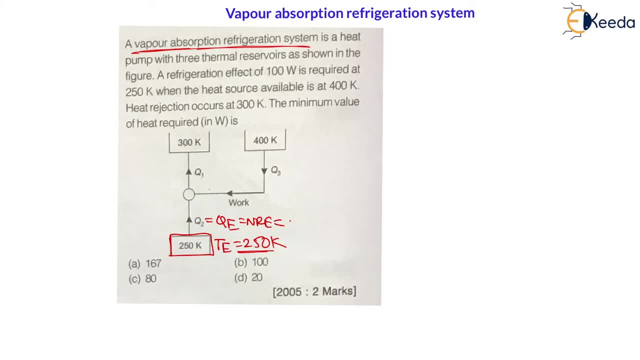 also called net refrigerating effect, which is given 100 Watt. 100 Watt, right, then. refrigeration effect of 100 Watt is required at 250 Kelvin when the heat source available is at 400 Kelvin. now, my dear students here, heat source is available at 400 Kelvin and the heat source is in generator, because generator 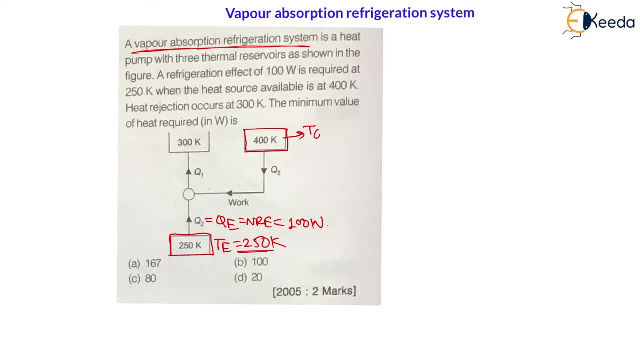 was supplying heat. therefore this is a generator. therefore, we can say: temperature of generator is equal to 400 Kelvin, right, and this Q3 will be heat of generator. we can say heat of generator, then heat rejection occurs at 300 Kelvin and, my dear students, heat rejection is always. 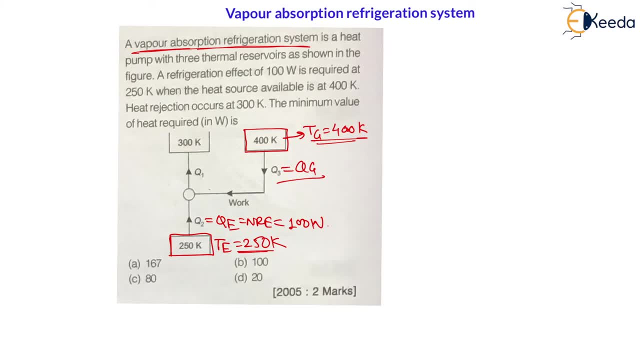 to the surrounding. therefore, this 300 Kelvin is nothing but temperature of surrounding. therefore, T0, temperature of surrounding. T0 is equal to 300 Kelvin right, and heat rejection to the surrounding is Q1 right now. the minimum value of heat required in Watt is now there are. 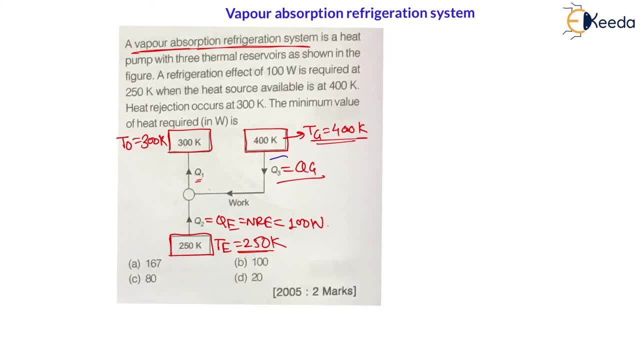 asking: what is the minimum value of heat required? the heat required is nothing but heat of generator. now, these heat in Watt, they are asking: what is the requirement? right now, my dear students, here we have got TE, Tg and T0. so, my dear students, the COP of this vapor absorption refrigeration system is: 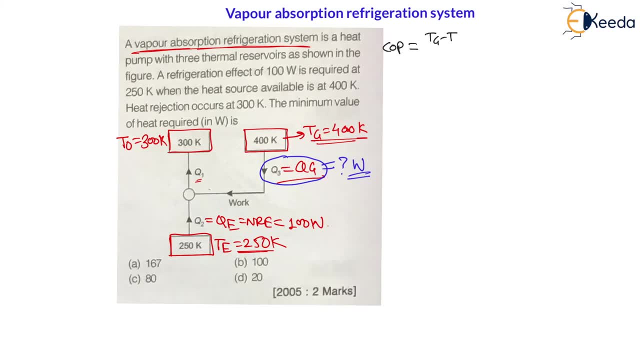 But we have just seen Tg minus T0 divided by Tg into Te, divided by T0 minus Te. This is the formula to find COP of vapor absorption refrigeration system. Therefore this COP will become Tg is 400 minus T0 is 300. divided by Tg is 400 into Te. 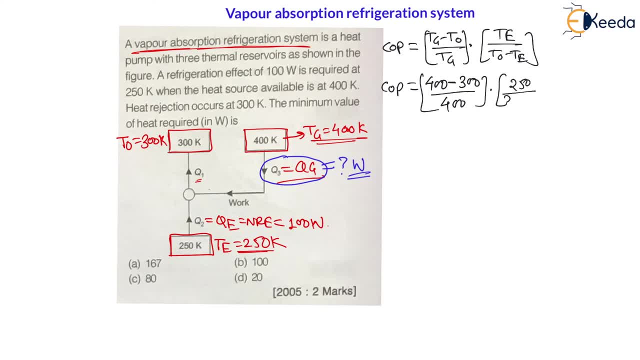 Te is here. 250 divided by T0 is 300, minus Te is 250.. So, my dear students, the COP of vapor absorption refrigeration system we will get here. This is 100 divided by 400 into 250, divided by here 50.. 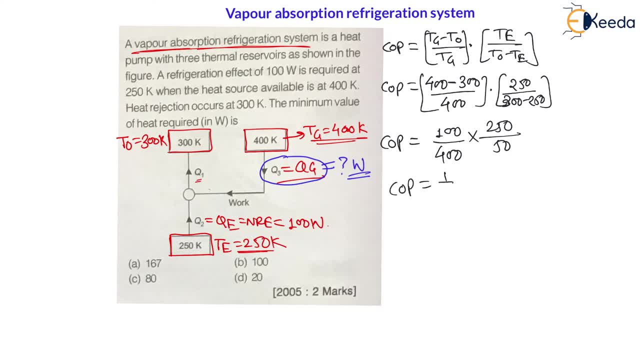 Therefore, if I find this, the COP of the cycle will be 1 by 4. into here, 25 divided by 5 is nothing but 5.. Therefore, it is 5 by 4.. The COP of this cycle is 5 by 4.. 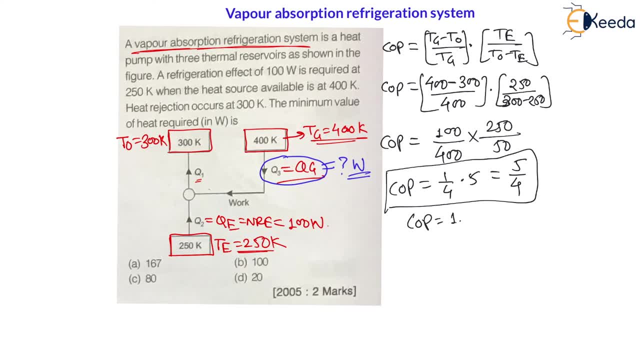 So, my dear students, therefore, this COP will be equal to 1.25.. COP of cycle is 1.25.. Now, my dear students, this COP is nothing but heat of evaporator. Do you have a heat of generator? 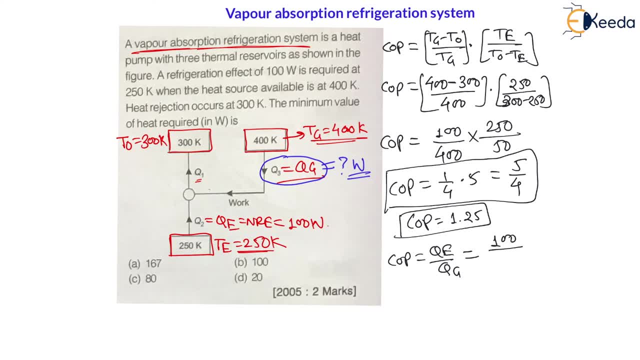 Therefore, which is equal to heat of evaporator is given 100.. Heat of generator is heat of generator. we have to find which is nothing but COP, which is nothing but 5 by 4.. Therefore, my dear students, if I find, 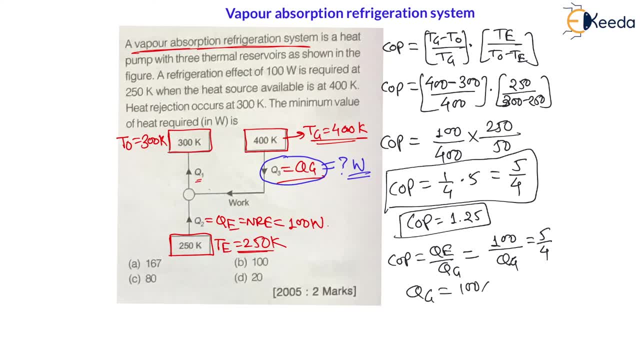 Heat of generator then I will get. it is 100 into 4 divided by 5, which is nothing but 80 Watt, 80 Watt. Therefore, the minimum value of heat required is 80 Watt. Therefore, this heat of generator required is 80 Watt. 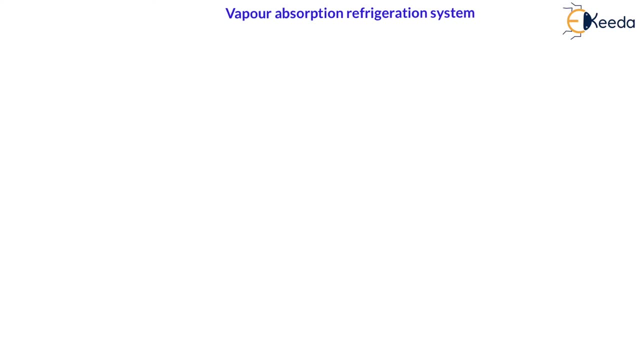 Therefore, answer for this question is option C. Now, my dear students, the one of the application of this vapor absorption refrigeration system is that it is used in Electrolux refrigeration. right Now we can say: in Electrolux refrigerator, in Electrolux refrigerator. this Electrolux refrigerator functions on the principle of vapor absorption refrigeration system, right. 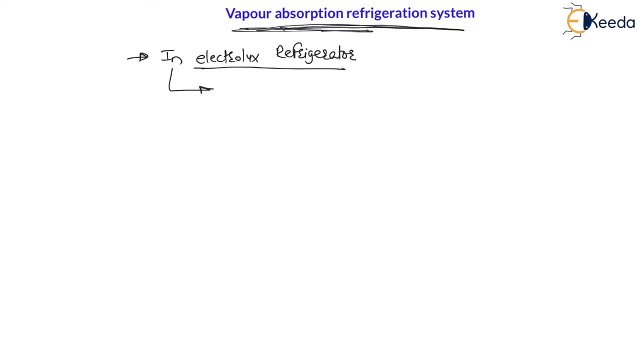 Therefore, but, my dear students, in this Electrolux refrigeration, the difference between vapor absorption refrigeration system and Electrolux refrigerator is that In Electrolux refrigerator there is no pump. pump is not used, and as pump is not used, then it is the operation is noiseless. the operation is noiseless means less pollution of noise, right? 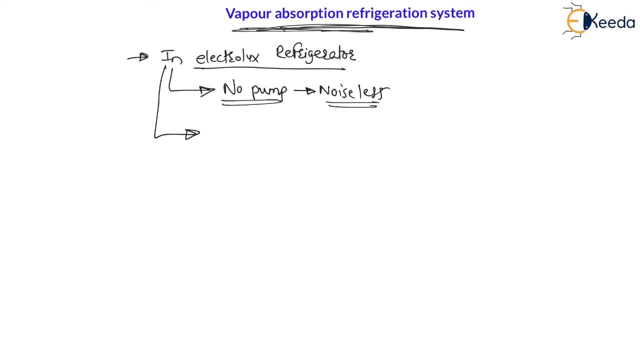 And my dear students, again, one more difference between vapor absorption refrigeration system and Electrolux refrigerator is that in case of vapor absorption refrigeration system, ammonia, which is refrigerant, and water, which is absorbent, is used. But here, In this case, that is, in Electrolux refrigerator, here ammonia is used as a refrigerant, ammonia is used as a refrigerant and same water is used as a absorbent. same water is used as a absorbent. and, my dear students, we have seen, in case of vapor absorption refrigeration system, the pressure reducing wall is used and the purpose of pressure reducing wall was to pass weak solution of weak liquid, solution of 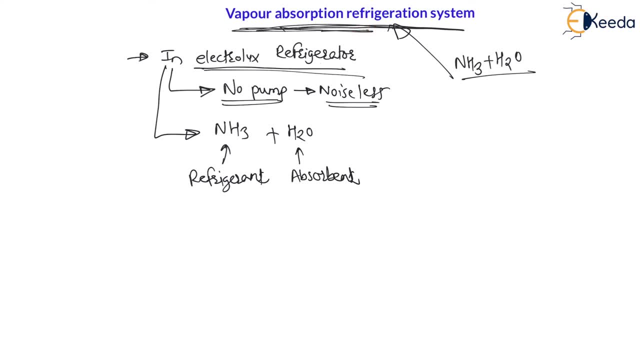 Ammonia and water back to the absorber. that already we have seen. this pressure reducing wall is connected between generator and absorber and, whatever may be the liquid refrigerant present in the generator is again passing through the absorbent through the pressure reducing wall. 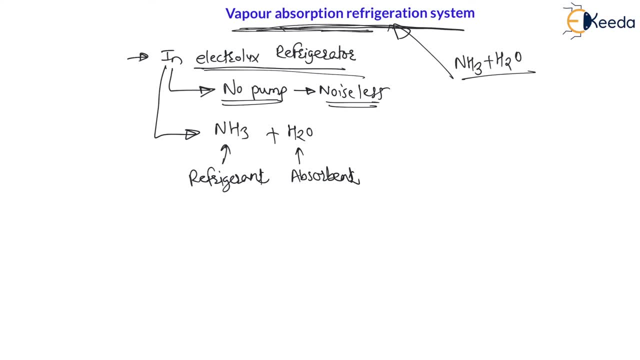 But here there is no pressure reducing wall. here hydrogen is used. here hydrogen is used to reduce the pressure. this hydrogen is used. it is used To reduce the pressure. we can say to reduce the pressure. The purpose of this hydrogen used is same as that of pressure reducing wall in case of vapor absorption system. 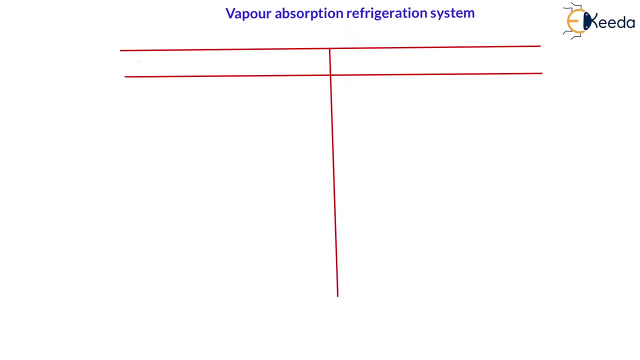 Now, my dear students, let us understand the difference between VCR cycle, that is, vapor compression refrigeration system, and vapor absorption refrigeration system. Now, already we have seen, in VCR cycle, compressor is used. In VCR cycle, compressor is used. 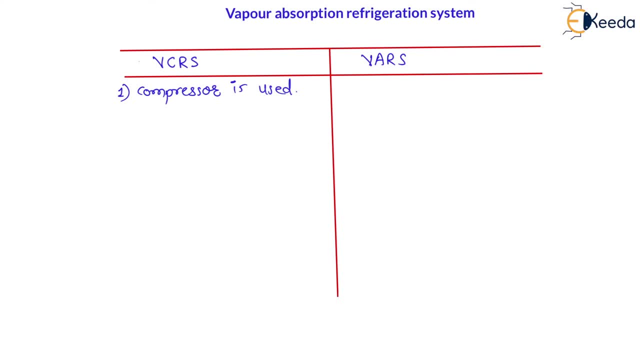 And compressor is electric And in VCR cycle compressor is used And in VCR cycle compressor is used. Therefore lot of electricity is consumed in VCR cycle. Therefore it is costly. Right The cycle will generate more electricity cost. 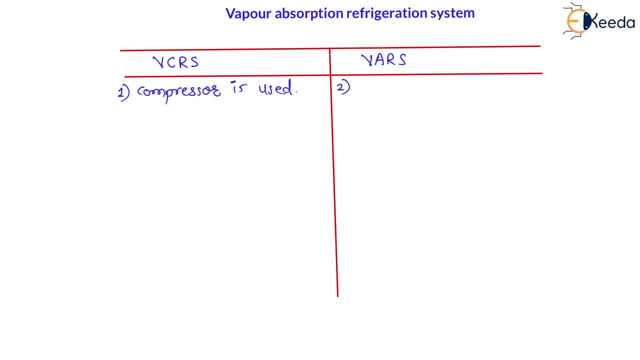 But, my dear students, in vapor absorption refrigeration system the compressor is replaced by. right here, compressor is replaced by: we can say: first is absorber, then pump and then generator. The same compressor, in case of VCR cycle, is now replaced with: 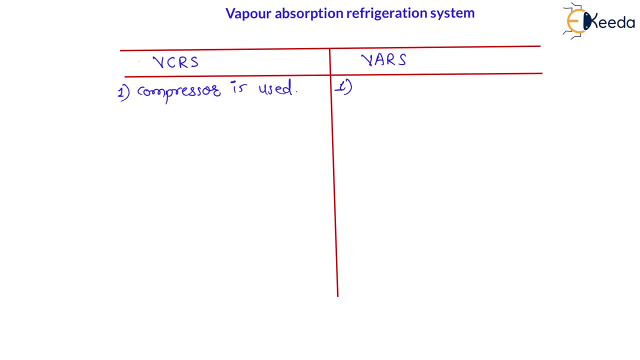 Right Generator, absorber and pump. Absorber, pump and generator is used. Generator is used in vapor absorption refrigeration system. Right Now again we have seen in case of vapor compression refrigeration system, COP was heat of the operator divided by work of compressor. 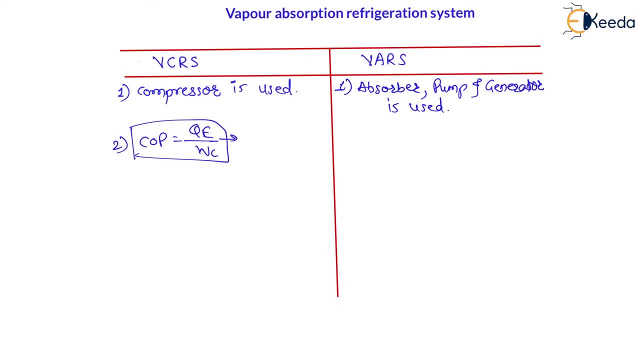 Means. work of compressor is the input here. Therefore it is work operated unit. We can say it is work operated But, my dear students, in case of vapor absorption refrigeration system, COP is nothing but heat of the operator divided by heat of the generator. 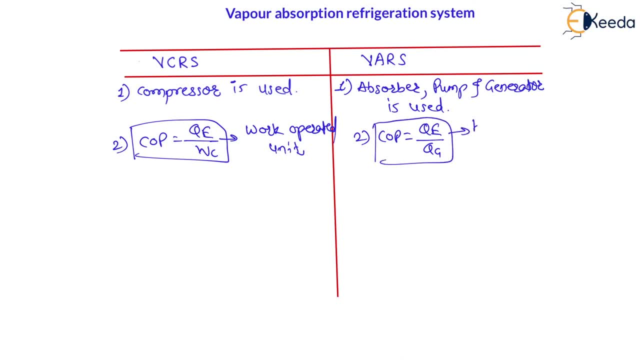 So, as it is a ratio of heat to the heat, therefore it is a heat operated unit. It is a heat operated unit Right Now. third difference is that the COP of VCR cycle is generally, my dear students, very high. 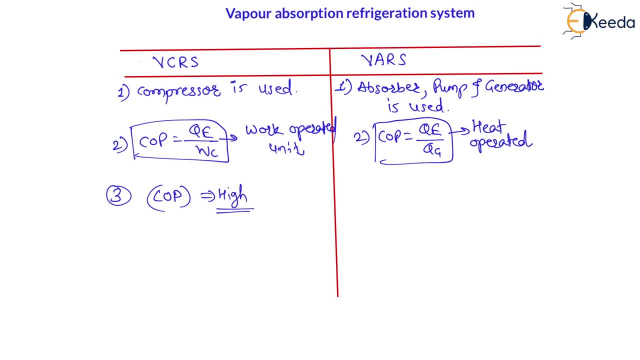 COP is high. Right, In case of vapor compression refrigeration system, COP is very high. And, my dear students, in case of vapor absorption refrigeration system, COP is generally low as compared to VCR cycle, Because here heat is used and here work is used.